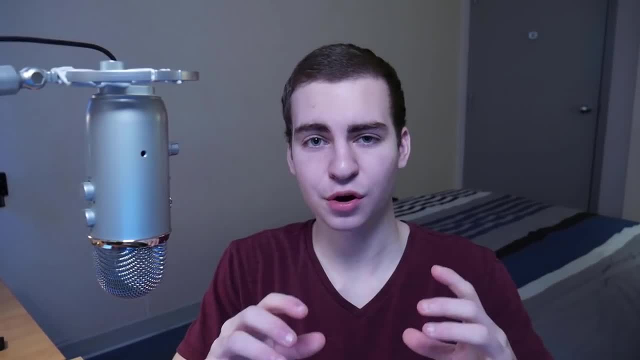 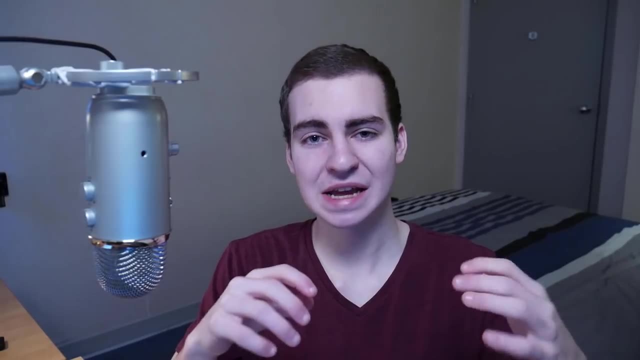 they're sponsoring this video- for me to talk to you guys about a new project they've started called the Microsoft dev collective. Now, this is a really exciting and great opportunity for you guys And essentially, I'm going to be talking to you guys about a new project they've started. 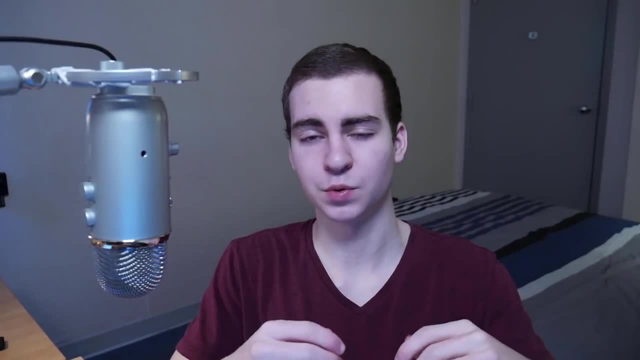 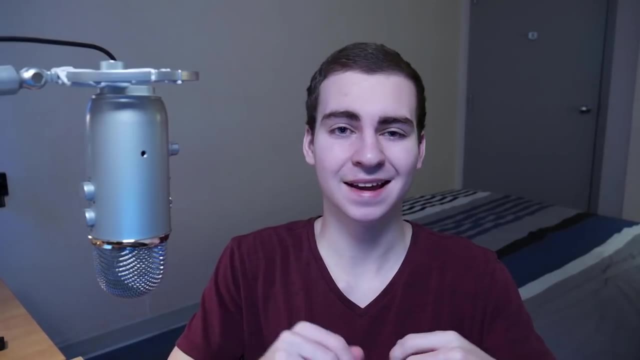 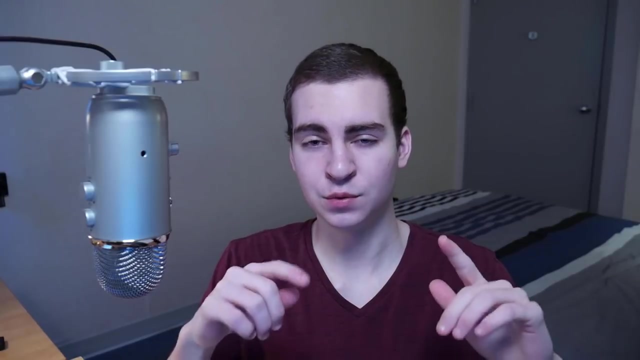 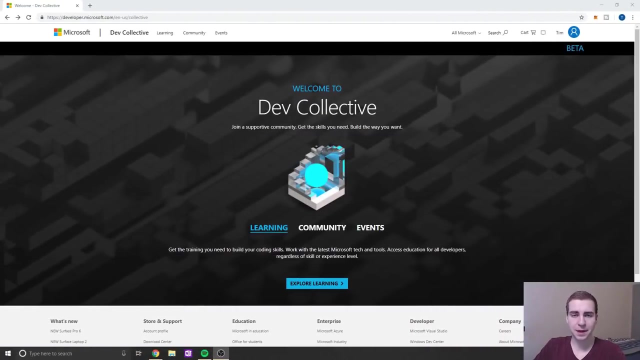 and essentially I'm going to be talking to you guys about a new project they've started called the Microsoft dev collective, And if you go there, it's going to bring you to a page that has a bunch of courses that look just like this. Let me show you. Okay, guys, so I'm on the Microsoft dev 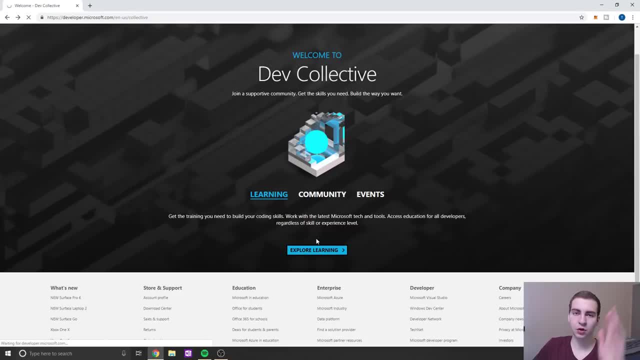 collective website. here I'm just going to click on explore learning and have a look at all of the different courses that they've provided, And I'm going to go to the Microsoft dev collective website here And if you go there it's going to bring you to a page that has a bunch of courses that 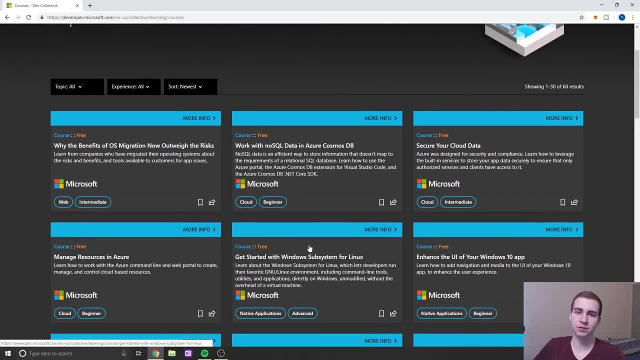 they have to offer as of now. So, like I mentioned, this is a brand new thing And there's going to be new content added on here monthly. So make sure you guys are continually having a look at this, Because since the first time I looked at it, there's been some new courses And I know that. 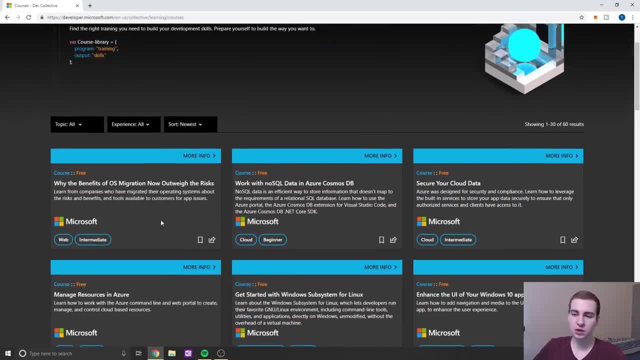 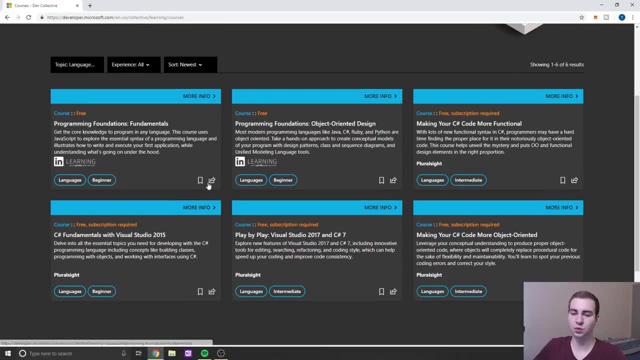 they're adding a lot of different content. that's going to be super valuable. So I just signed in here so I can gain access to all these courses, But essentially I'm going to go to topics and just go to languages And this is where my tutorial will be showing up And essentially, you can have 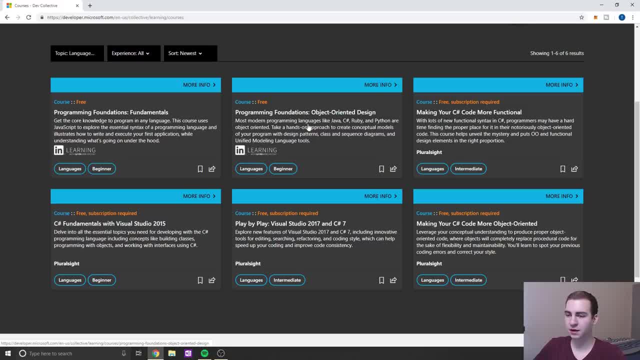 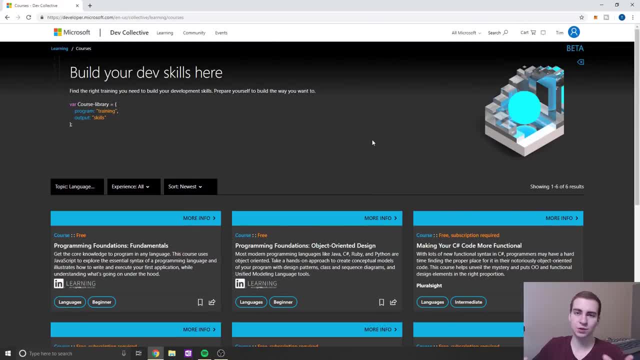 guys have a look at here, you're probably going to find something that interests you And it's free, So what's the harm? and having a look at it and checking it out? So, anyways, that's been it for this little ad thing. I hope you guys did listen to this And I hope you're going to get some value. 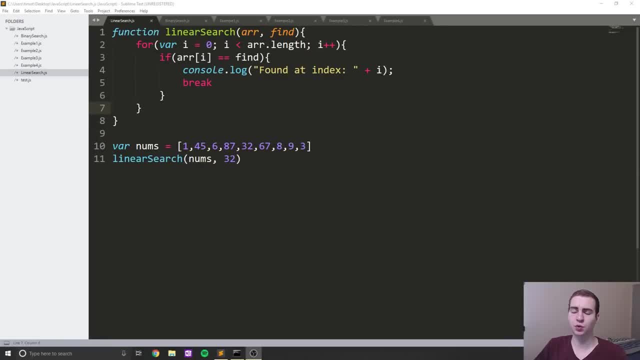 from this and now on to the video. Okay, so what this tutorial is really going to focus on is time, complexity and big O notation. Now, I'm not trying to make you guys pros in this, But I really want, by the end of this video, that you guys are going to be able to look at certain algorithms. 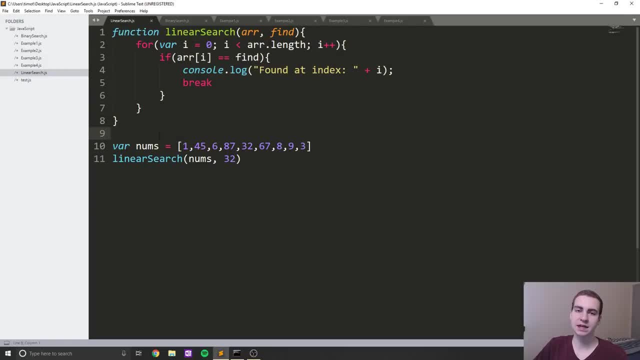 maybe something that looks like this: analyze them and get some kind of idea of how long it's going to take for them to run. Now this is a really important skill. It's taught a lot in computer science in general. I don't really care if you guys know how to do like big O of n or n. 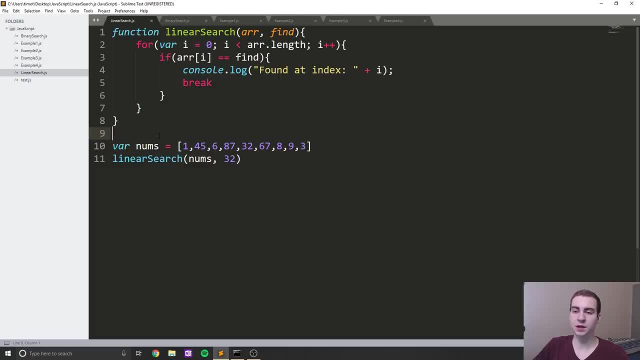 squared or like n plus one. I just want practically you would be able to look at an algorithm and be like: okay, so like, based on my knowledge of kind of time, complexity and how things work, this is going to take a long time to run And the reason why that's really important. 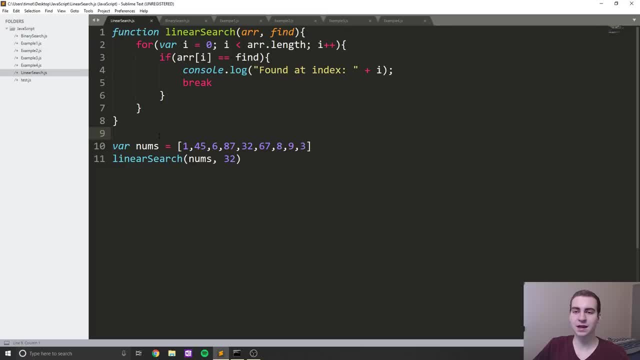 is because when you guys are writing code- I see it a lot with beginners- they have no idea about how long it actually takes for something to run And if you're trying to run things on like 1000s and 1000s of lines of input or less massive. 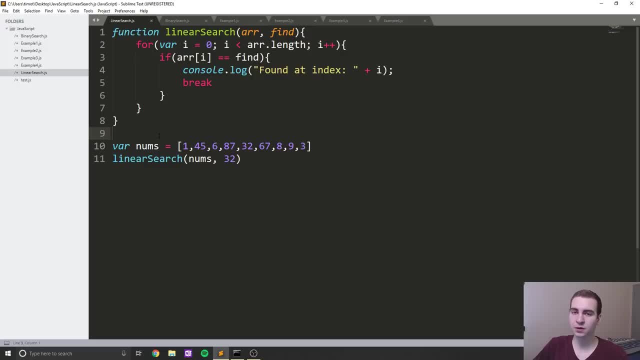 I don't know, like text files or something like that, and you have a really inefficient algorithm or inefficient code. it's going to take forever and it might not even run. So I just want you to be conscious of the fact that your code really has an effect on how long it takes for the computer to 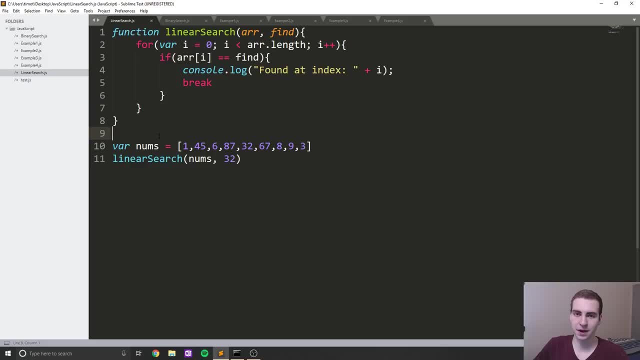 execute something, And typically the faster something is, the better. Now we're going to talk about it. A bunch of different algorithms here that I've personally just wrote myself. some of them are, like, very well known, but I've just created a few, And I'm going to be doing this in JavaScript, But it 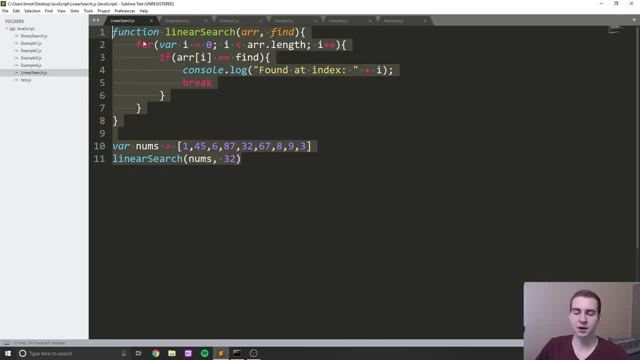 doesn't really matter if you don't know JavaScript, because this is just. I'm not going to be writing any code, you're not going to be, we're just going to be analyzing it. So as long as you can kind of get an idea of what this code is doing and you've programmed before, you're gonna have no problem. 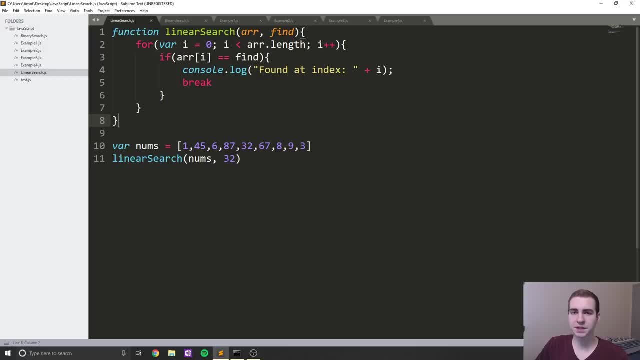 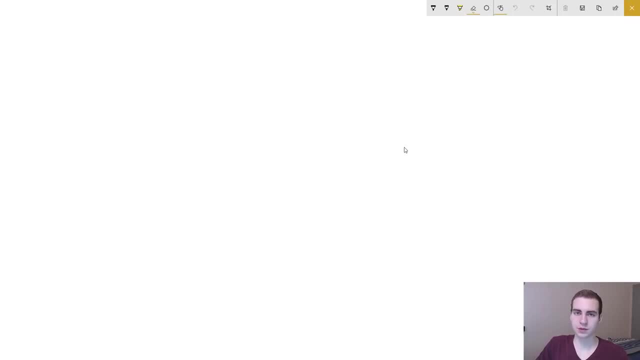 following along with this if you don't know JavaScript. Okay. so, with that being said, let's get started And let's talk about bigger notation and time complexity. Okay, so, what is big O notation? Well, bigger notation. Why is this not drawing on the eraser? That's why bigger. 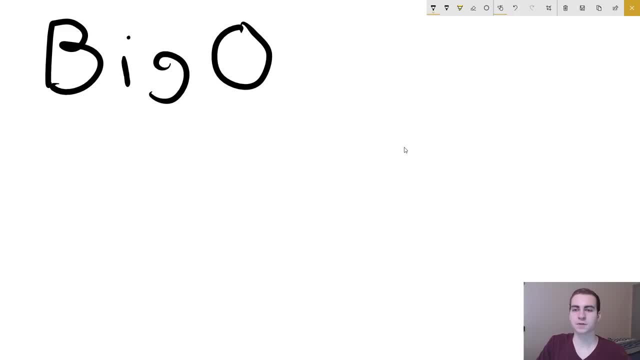 notation is essentially just a fancy word or fancy notation for denoting how long it takes for a certain algorithm to run. So I've already said algorithm like 100 times, but that's what we're going to be focusing on: algorithms. Now, what is an algorithm? essentially, an algorithm is a set of 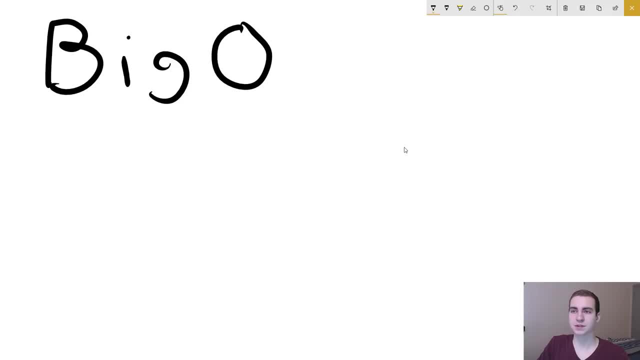 instructions And typically in computers, based on some input, it takes like a certain amount of time to execute, And that's what we're really going to be focusing on here. So, algorithms, set of instructions, big O notations: how long does it take this set of instructions to run based 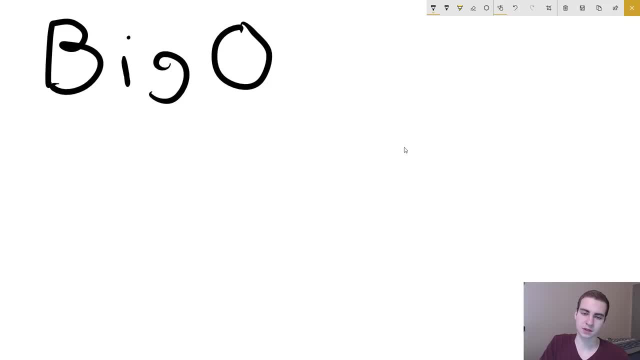 on some kind of input. So what we're mainly focusing on here is input. Okay, so in a specifically input size, and then that's going to be related to time. So, based on some kind of input size, how much time can we relatively expect this algorithm to take? Now, I'm not saying we're going to measure it in. 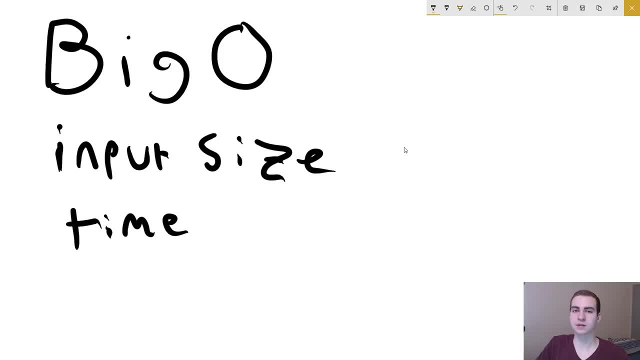 seconds. we're actually just going to measure it in like relative operations, And what I mean by that is like an operation could be something like adding one to a number or like grabbing information from an array. That's how we're going to measure it in amount of operations, because 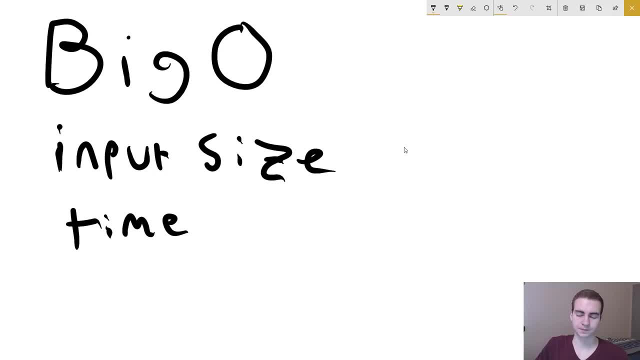 obviously based on different computers, things are going to run a different time And there's a ton of different factors that affect the actual time. But we just want to get some kind of idea, like: are we going to sit here for hours Or is it going to happen in a few seconds, And that's the main? 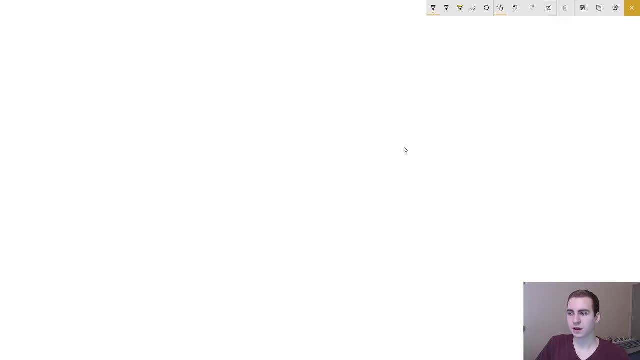 idea of big O notation. Now, quickly, before I go on, something that's important to understand is that when we talk about big O notations, we're going to talk about big O notations, And that's something that's important to understand is that when we talk about big O notations, we're going 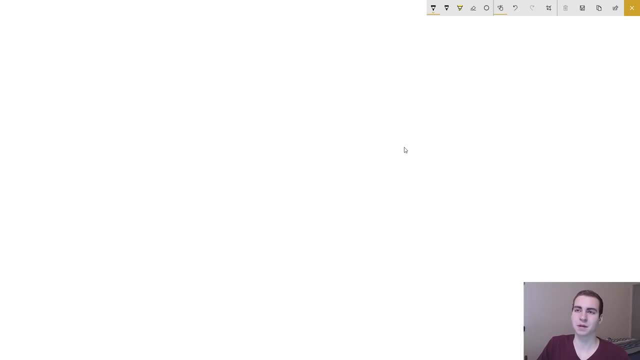 to talk about big O notations. we're typically talking about very large, massive amount of information. Now, what I mean by that is, for example, if you have an algorithm that needs to run something on like five numbers- okay, let's say we have like 12345, like this: our list, okay. 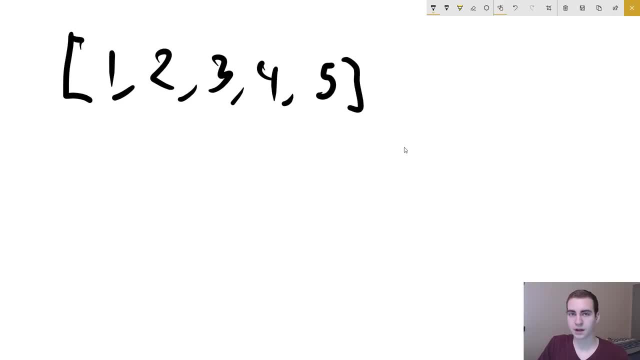 you need to do something with this list. Well, computers are super fast, like they can do 1000s of operations per second. So if we have an algorithm, it's like pretty inefficient, but we're only taking like I don't know, we're only using like five elements, like we're not going to be. 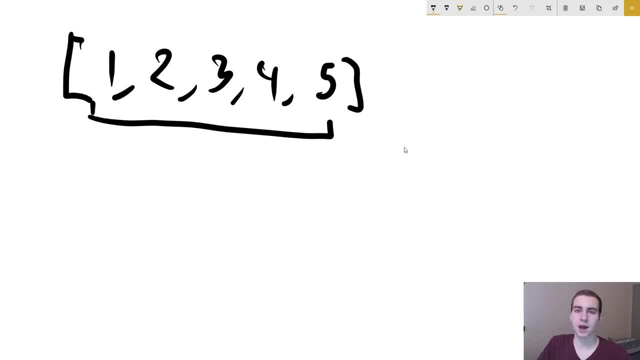 using that algorithm. very often we just then. it doesn't really matter how inefficient it is, because it's still going to happen almost instantly. You know what I mean. It's like if you write one line of code and it. 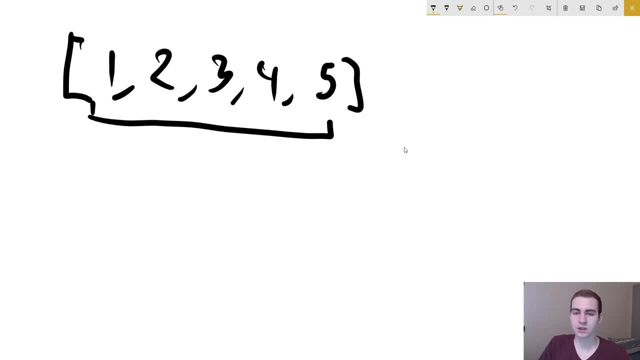 could have been replaced with like five. that was a lot faster. Well, if we're only using like a really small amount of input, it's kind of negligible because you're saving like maybe like a millisecond right. So it's almost just. we don't really care about small data sets, we only 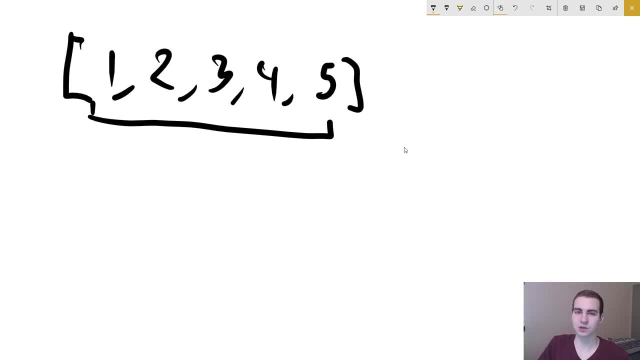 care about large data sets, And you guys will see what I mean as we go through here. okay, So now I'm hoping you guys have a little bit of a math background, because I'm going to start kind of just drawing some functions here and talking about growth And yeah. so what we're going to do is I'm 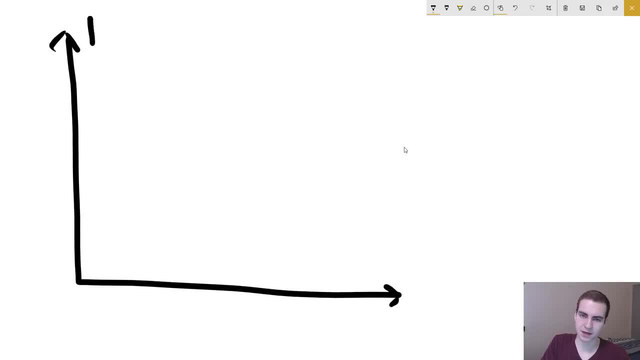 going to draw two axes here, Okay, and I'm going to call this my time axis. Okay, And this is going to be n. Now, I haven't talked about n yet, So that's what we're going to do now. So, essentially, 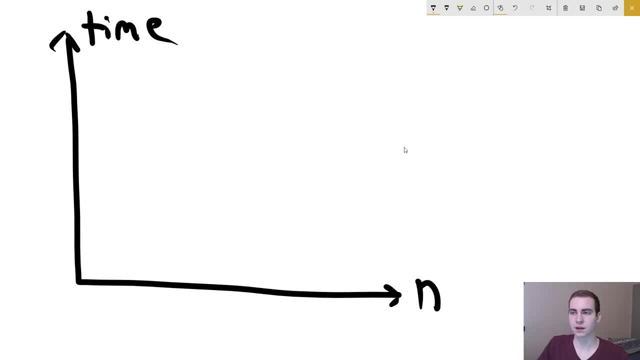 remember I was talking about. we only really care about large data sets or like large amount of information. essentially, we're trying to figure out, based on some kind of input, How long is our algorithm going to take relative to that input is going to take like five times. 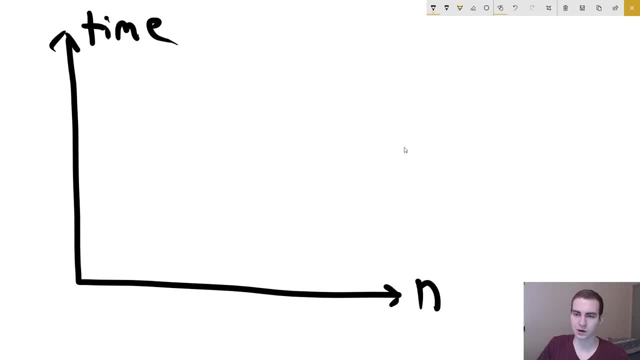 that input, like, how many operations is it going to do on that input? that's what we want to know. So our input, like if we have, let's say, an array, okay, the length of that array is going to be noted, denoted by n. So n you're going to see me use this a lot- This just means the length of the. 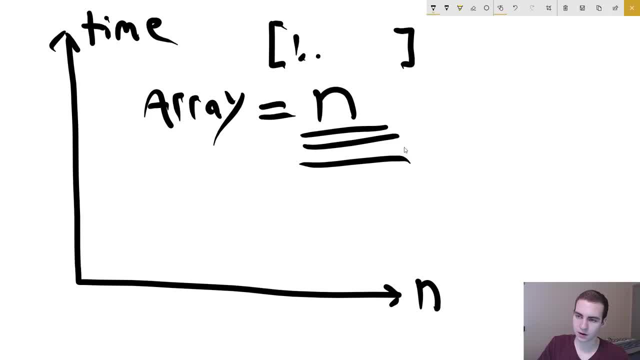 array. So if we have an array like this, we go from one comma- dot, dot, dot- to n, So the length of this array is n. That's really important. We're gonna be, that's gonna be brought up a lot, So let's get rid of all. 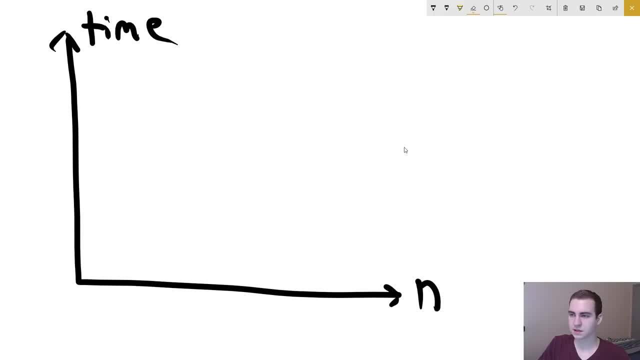 this. Now, This eraser is not that easy to use. Okay, there we go. So, based on some kind of input, and we're gonna be figuring out how many operations- in other words, like how much time is it going to take us to run- So I'm just going to draw two functions on here And I want you guys. 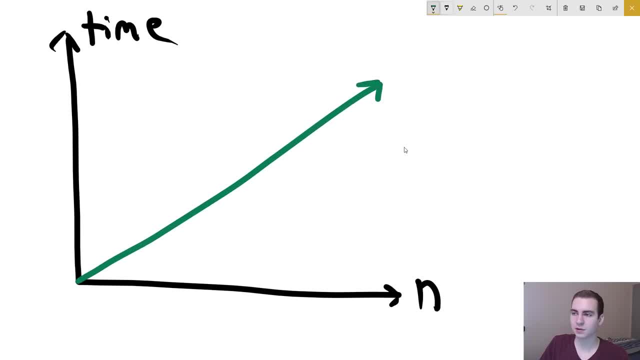 just to think about which one you would rather have. Okay, keep in mind, everything we want is like super efficient, like that's what we're aiming for. Okay, so let's draw this And let's draw a purple one that looks something like this. Okay, so we kind of have these, this intersection. 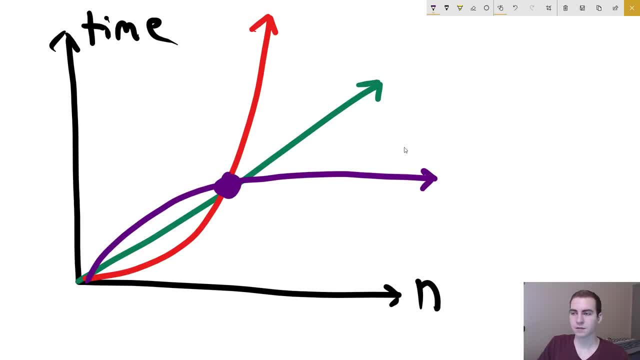 point here at this purple dot. But these are three different functions. Now if you guys know anything about math, you should know what these functions might be. So, for example, this function could be something like time equals n. this function can be something like time equals log of n And this: 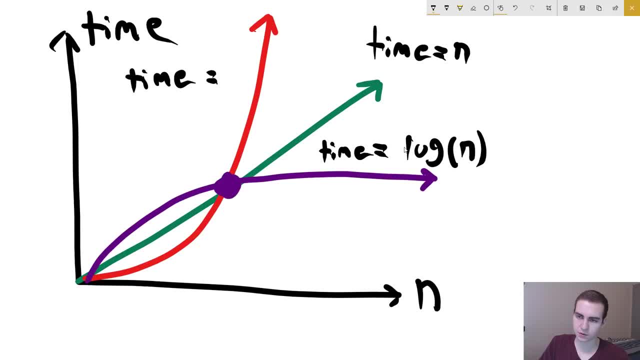 function could be something like time equals, and then maybe something like n squared okay, like a quadratic function, which would mean it would go like that too, But we're not, we don't care about the negative side. Okay, so three. 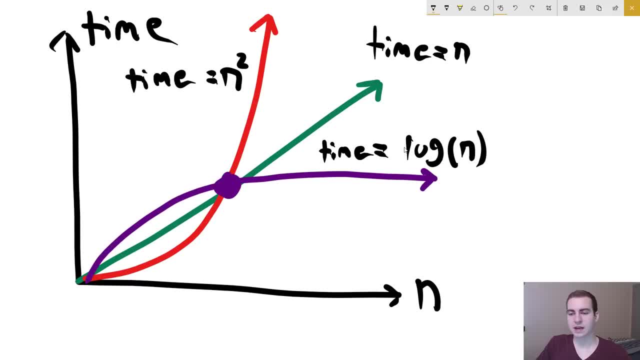 different functions. Now I'm going to ask you: if you're running an algorithm and you want it to run as fast as possible, based on, like, massive amount of input, which function would you take? like, let's say, these are three algorithms, these are how long they take. Do you want this one? Do? 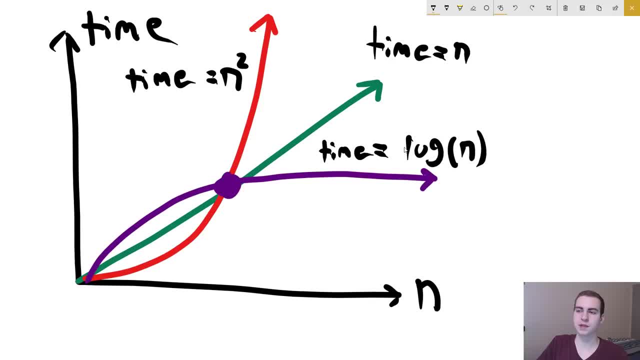 you want this one, Or do you want this one? For how much time they're going to take? just based on their graphs, expecting that this is going to take a lot of time. So let's say that this is going to continue on to infinity right. Which one would you want? Well, I would hope that you guys would. 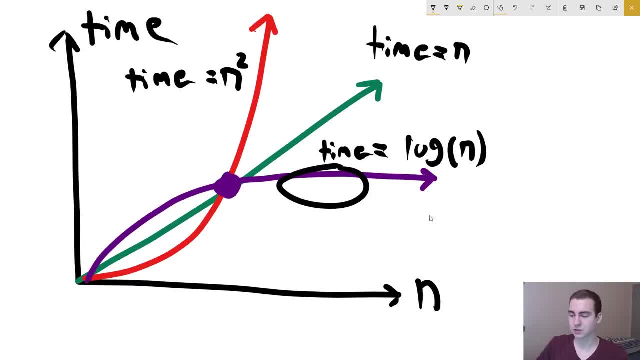 say this purple one right, that you guys would want this purple function which is login. Now, the reason you'd want that is obviously because, as the size of the input increases, the time is very slowly increasing. Like, look, have a look at it here, right? So at the beginning it increases. 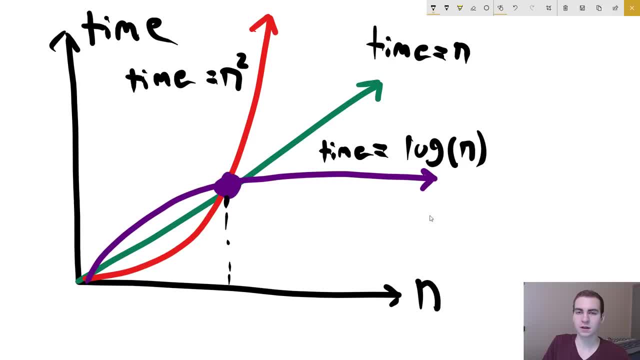 faster than all the other ones. But once we get to this point here, it starts slowing down and the slope is actually decreasing as we continue to go. Alright, let's have a look at the red one in comparison. Well, the red one is actually way it's. it's faster up until this point, right, Because the time is. 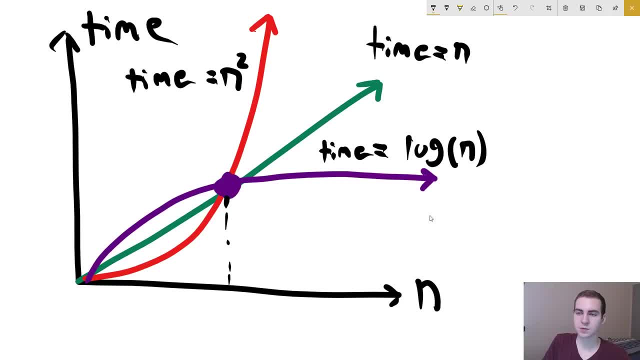 is slower, But as soon as we hit here you can see it starts exponentially increasing, increasing, increasing and keeps going. And this green one, well, this one's fine, but it's just a straight line, it's linear, So essentially it increases at the same rate the entire time. based on n. time is. 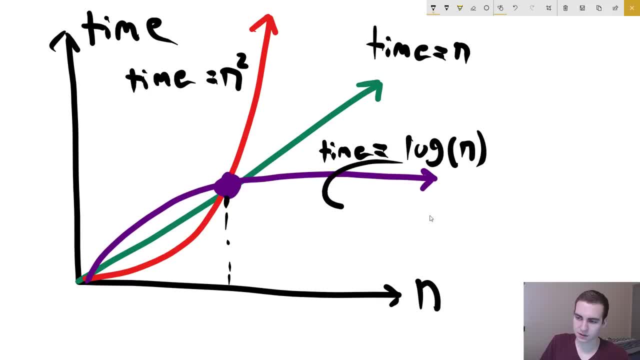 going to be exactly n right. So just, we want this, this log n. Now some people would say, though well, what if our input size is like: let's say: this is like: n equals n right, So let's say that. 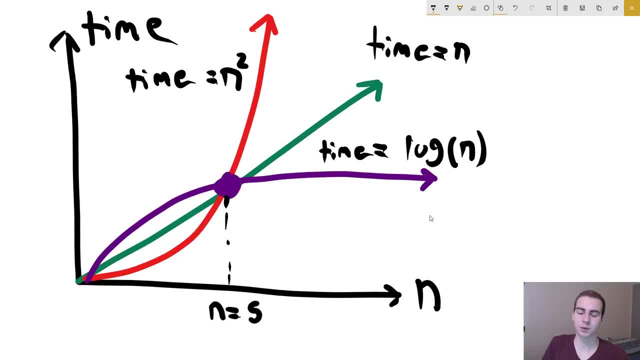 this is like n equals five. Okay, let's just say that's the number. I know it's not, But let's say that's the number. Well, if we had an input of like size three, so maybe like somewhere here which. 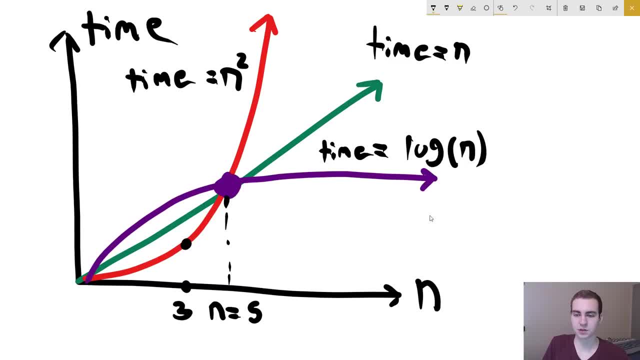 function would you want? Well, you'd probably want this red one, because the time is the shortest, But the thing is, yes, you would want that for the shorter amount of input, But as this input gets larger, larger, larger, larger, larger, you can see that this goes way faster. So that's why we 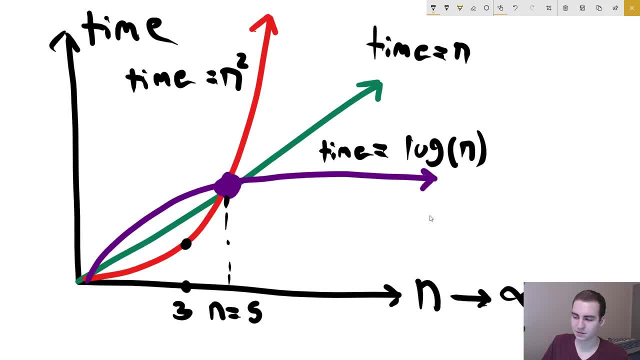 really care about when n approaches infinity, So when n is like a massive, massive, massive, massive number as opposed to anything on kind of the left side of this, like intersection point between different algorithms and different functions. I hope that kind of makes sense. This is the visual. 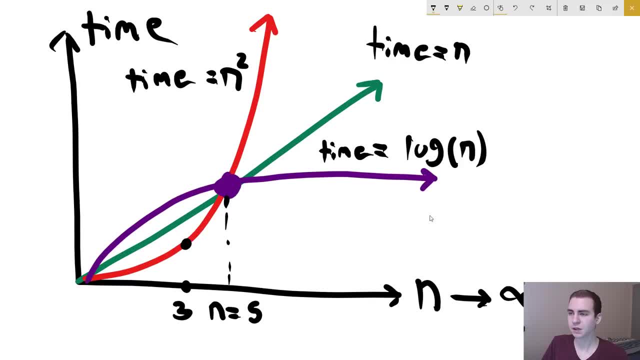 right of the speeds for our time. Okay, so we've just kind of found out now that log n right. this is: this is a way we're going to use big O notation with log n as well. We'll talk about that in a 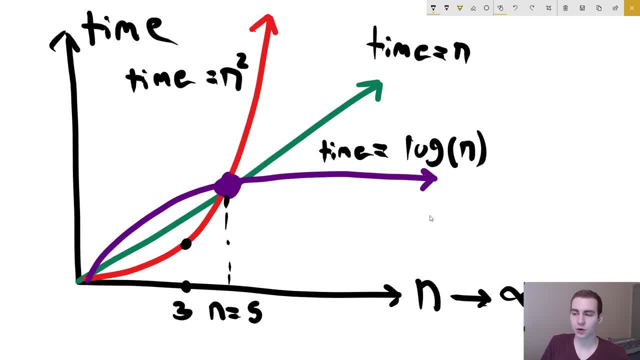 second is way faster. you can do way more operations with log n, then n squared right, or then time and not more operation. sorry, it just faster in terms of time. So these are kind of a few standard function times like how algorithms run in these certain times. Okay, so let's now start. I guess maybe. 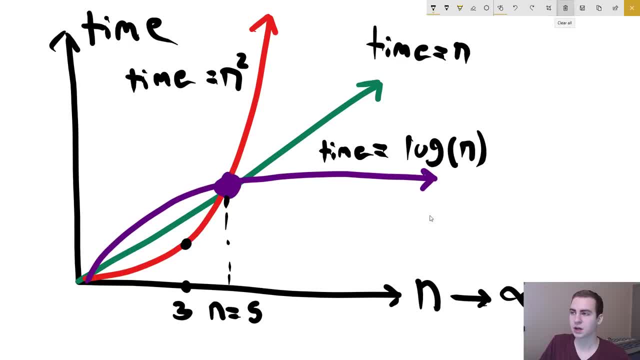 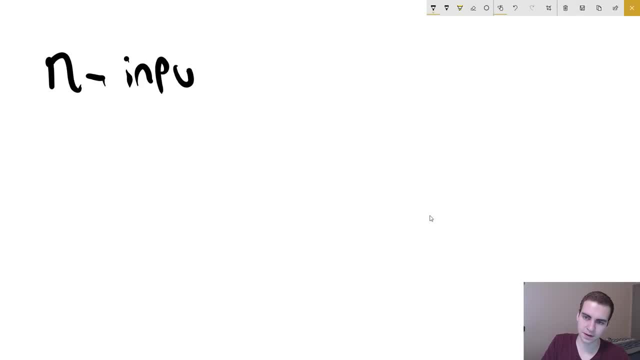 analyzing some algorithms, talking about how we actually write big O notation and stuff like that. Okay, so remember, I said our input size is n, so n is our input. Okay now, when we write big O notation. so we're trying to figure out how long something's going to take to run, or we know. 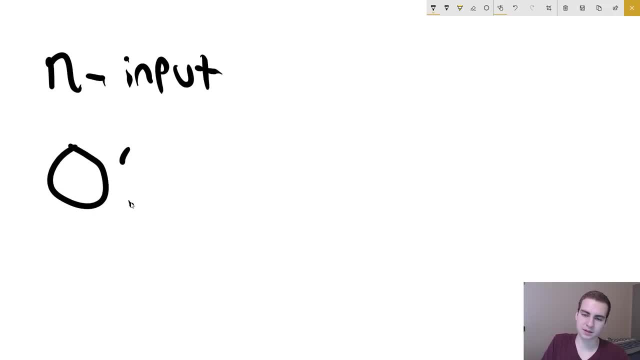 how long it takes to run. what we do is we write a big O, we put brackets and then in the brackets we put some kind of function based on our n. So the function could be like n plus one or n plus two. sorry, it could be like n squared it. 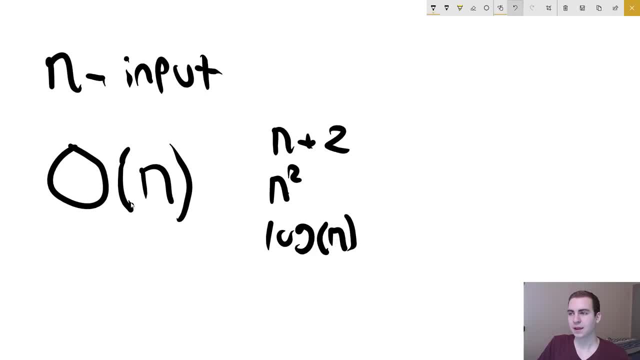 could be log n. it could be anything like that. Now remember how I was saying: we only really care about massive inputs, right? So when n approaches infinity? well, if you've ever done anything with limits, you'll understand what I'm about to do here. But let's say we have a function. 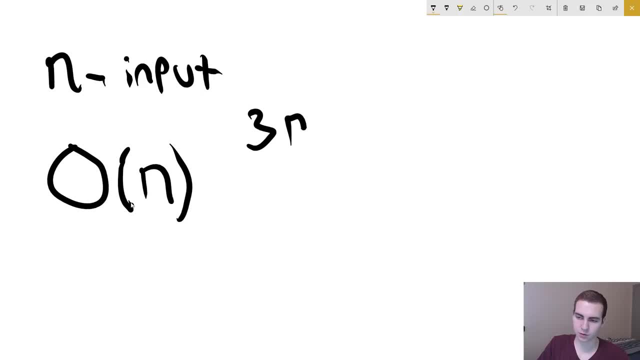 or let's say, the amount of operations that some algorithm does is like three, n plus seven. okay, like, this is the function. like, if I were to draw it, then we would have like a little grid. this would be seven, we would go like that. okay, that's what our function would look like. Now we only care about massive. 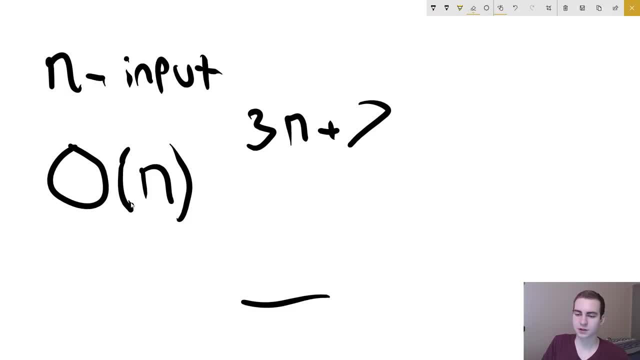 input sizes. So what we can actually do is we have a function that looks something like three n plus seven. we can actually simplify this, And what we can do is we can remove all of the constants. Now, what are constants in this? What's a constant? a constant is something that doesn't change, that stays the same. So let's have 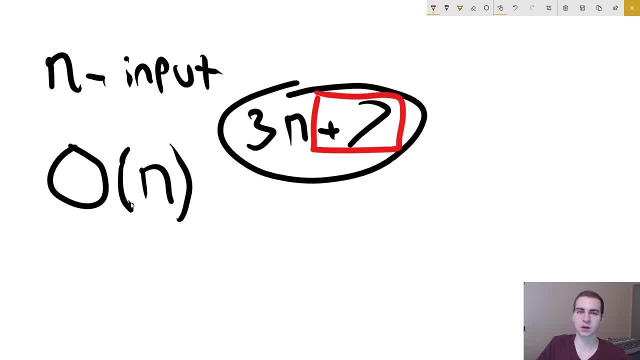 a look at this: this plus seven, This is a constant. So, essentially, whatever the size of n is so like, n could be infinity. we're going to do that times three. so three times infinity plus seven. Now, let's, let's think about this right. So n is infinity, because that's what we care. 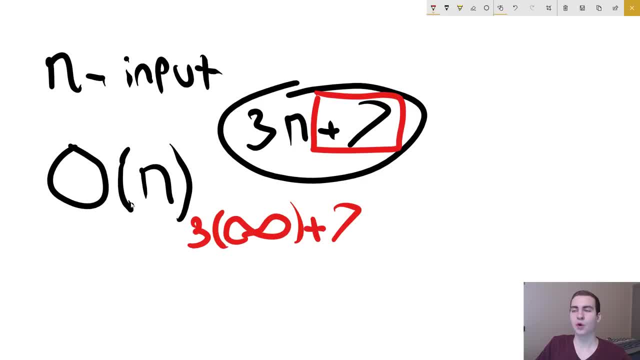 about massive inputs. does adding seven to infinity really change how long this is going to take? Like, imagine, imagine 10 billion, add seven to it. it's still pretty close to 10 billion. right Like that seven didn't really make a massive difference. So what we can actually do is we can omit this seven. 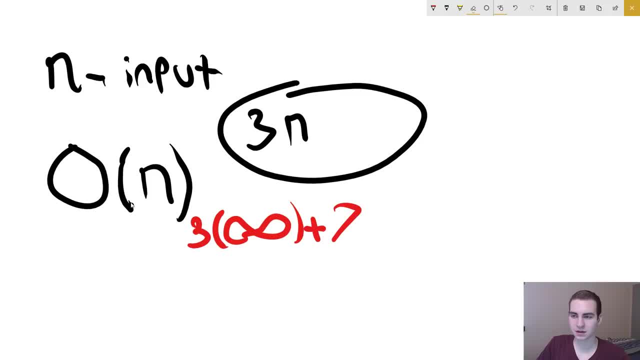 we can delete it. And why can we delete it? because it's a constant. even if the constant was something like like 10,000, we can get rid of it, we can delete it. And the reason we can do that is: 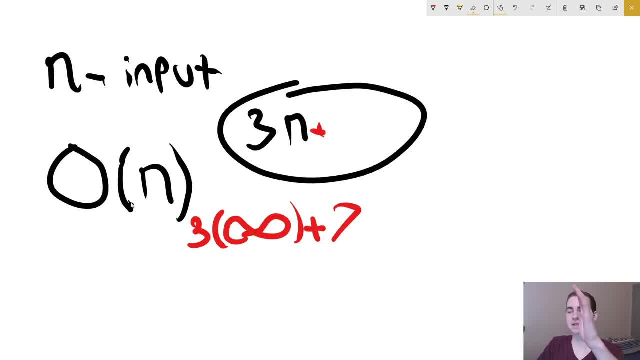 because we only care about the input size at massive numbers. So we can get rid of the input size at massive numbers. So we can get rid of the input size at massive numbers, So we can get rid of the those constants. Alright, so let's now we have three n. So what about? what about three? Is there? 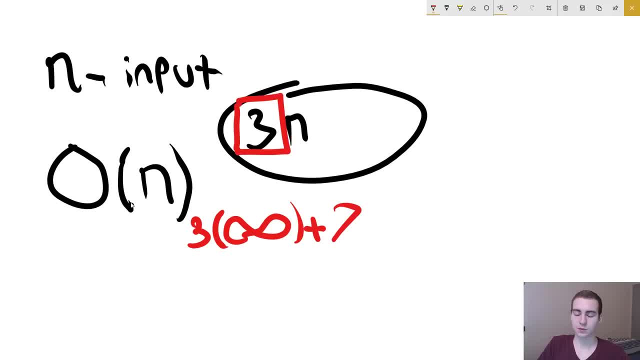 any other constants left. Well, three is actually a constant as well, And the reason it's a constant is because it's not a variable, like any number. that's not a variable is a constant or a function. So we have three. Okay, so this is a constant as well. So let's think about this now. So what we've? 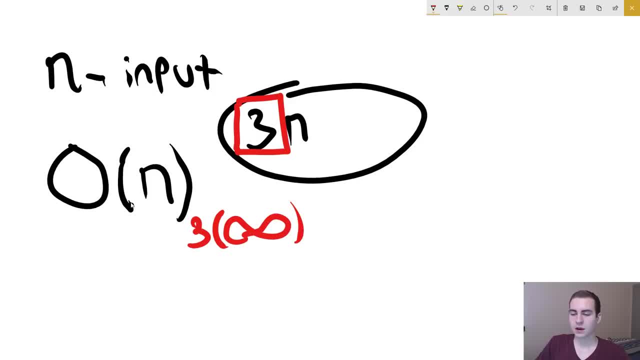 done is: we've simplified this to three times infinity. Now, three times infinity, what does that equal? Well, that actually equals infinity. three. anything times infinity plus infinity divided by infinity is still infinity, because it's just an arbitrary term. we don't really know. 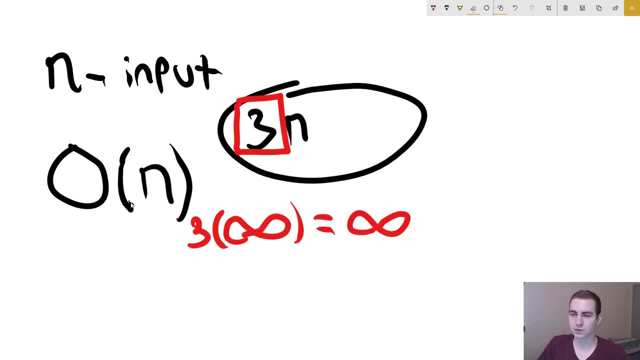 what infinity is. So what we can actually do is we can remove this three as well. So we went from a function that was three, n plus seven to simply n, Right. So if we compared them on a grid, we would have had this one, which was that original function, And now we have a function that looks: 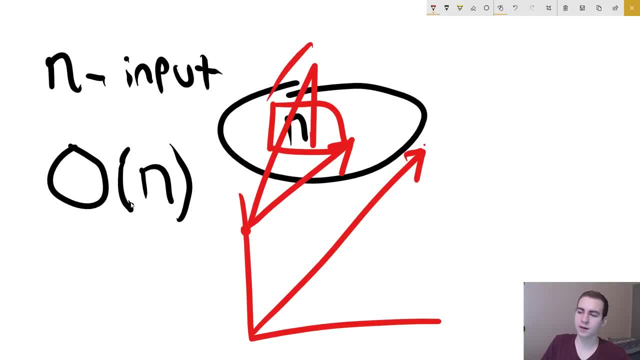 kind of like that right. So maybe this one had like a higher slope, like that, But now we have one that looks like this. Now the reason we can do that you're like: well, these functions are different. Three functions are different, But the thing is they're both linear, meaning that as n increases, 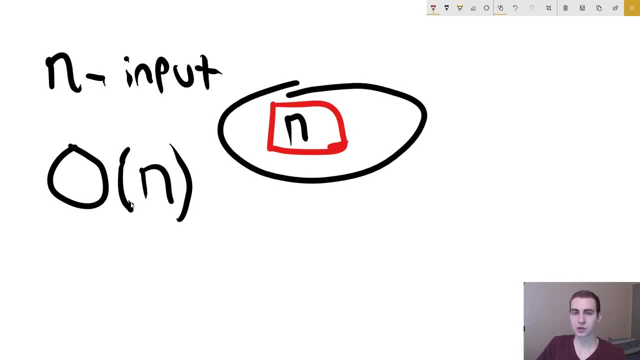 what do you call it? the time increases linearly, not exponentially. it doesn't grow any faster, it grows at the same rate, And that's what we care about. the rate of growth of our function. we don't really care about how like the exact number that it is, we just care if it's linear, if it's 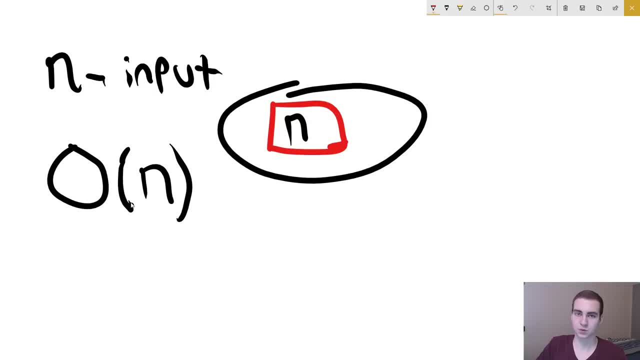 quadratic, if it's exponential, if it's cubic. that's what we care about, And we're going to go through a bunch of examples of different ones right now. Okay, So that's how we kind of simplify our things. we can remove the constants, meaning we don't really 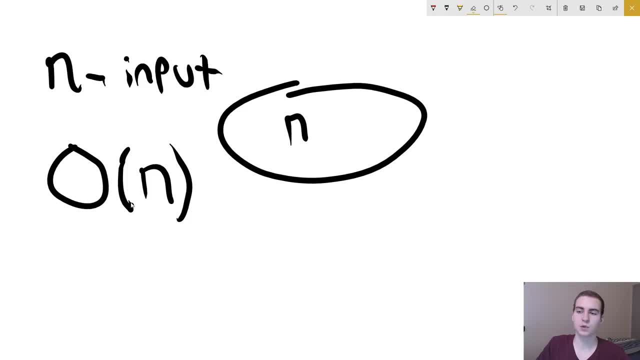 care about, like those plus 10s or those plus 15s And three times. we only care about the actual kind of variable value and what that means in terms of growth, So just the type of function, really. So let's do. let me just draw a few examples of some pretty common what do you call it? like big O? 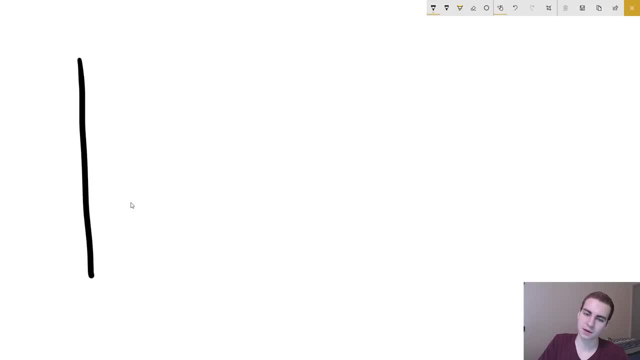 notations. there's some pretty common like runtime complexities. Alright, so let's do a grid, And we already did the linear one, right, right, we already did the log And we already did the quadratic, which looks like that. 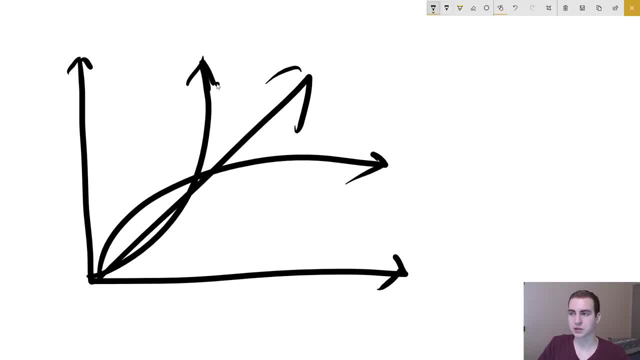 okay, these are three very, very common big O notations are like runtime analysis: that you're going to see a lot, And when we start going into actually analyzing algorithms, you guys should understand this a lot better. Okay, so those are three common ones, But 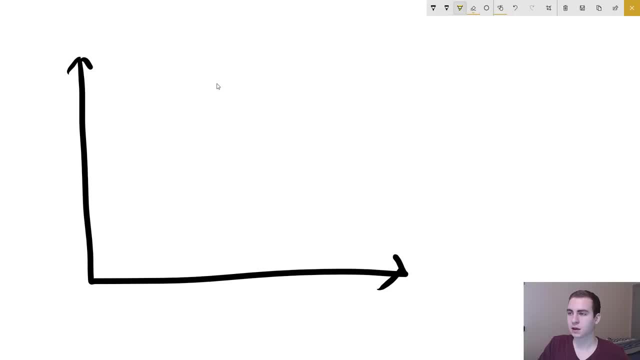 there's two more that we want to talk about, And we're going to rank them in terms of like how long they take, which one is slower, which one is faster. So we did log n, But what about? what do you call it? Let's see what about two to the n. So we did was we did n squared. 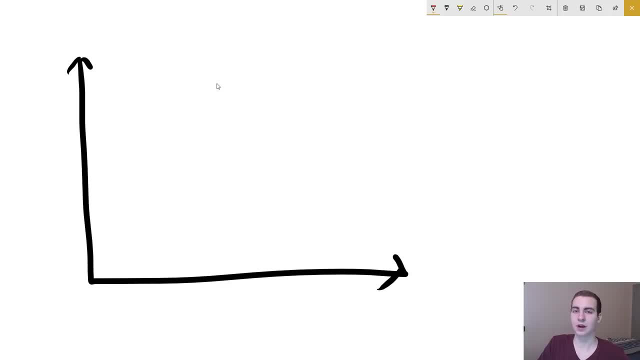 but we also did two to the n. So who knows what's faster to the n or n squared? Well, two to the n is actually way, way, way slower than n squared. So this is two to the n Okay. 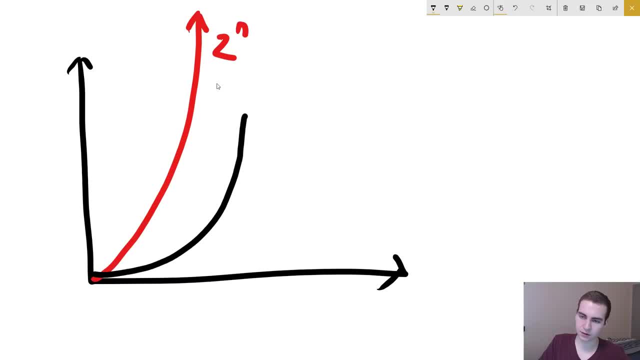 And if we do and squared and squared looks something like that, So they both grow exponentially, but two to the n grows way faster than n squared. So if I gave you two algorithms and I said: Algon, well, it's time it takes two to the n to run And I said: out to that takes n squared, which. 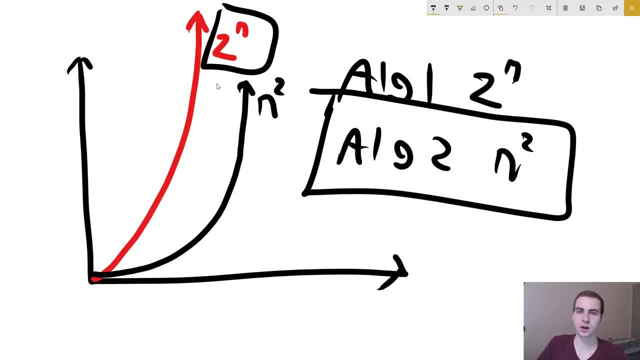 one would you pick? You'd pick n squared. Okay, so that's just important to understand, because a lot of people don't know to the end, although it seems like, Oh, and to the end is a way, it takes a lot longer and a lot more operations than n squared. I'm going 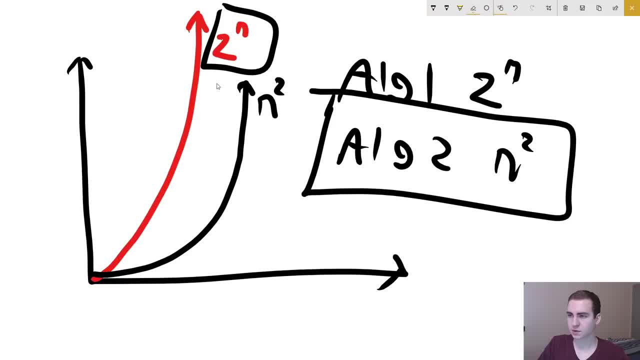 to show you an example of two to the n in a second as well. Okay, so there we go. So that's another example of one. Some other common ones. We can use more than one variable, So sometimes when we do algorithms, we might have more. 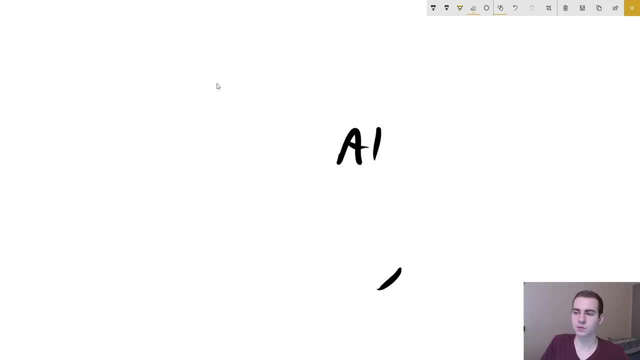 than one list or more than one, I don't know. input right, We can have two inputs, like say we have a function and it takes two inputs. So let's say we have an input and one, and we have an input and two. Now a common runtime analysis for two inputs is something like: 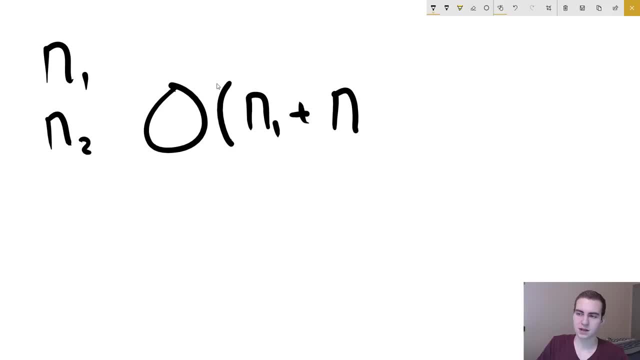 big O of n one plus n two. Now can we simplify this any further, Right? So remember, I was saying: like we have three, n plus seven, then we can just scratch out the seven. we can scratch out the three, we only care about. 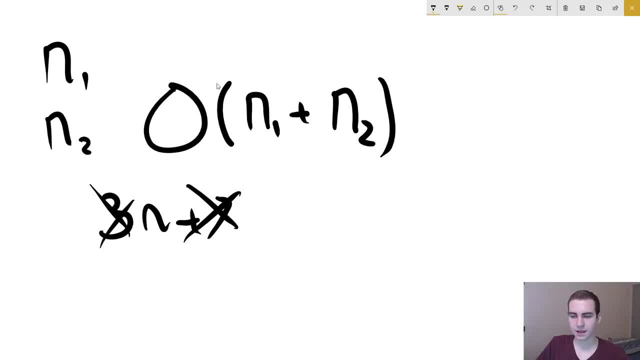 the end, because that's kind of the rate of growth, right. And then I guess we can do the same thing. If we have something like three and squared, well, we can get rid of the three And we'll just keep the n squared, because that shows us kind of the shape of. 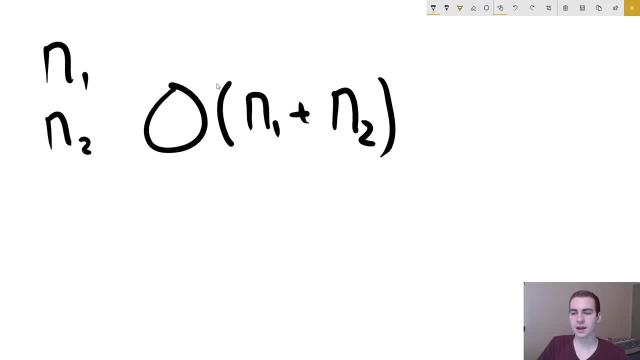 growth, which is what we care about. Okay, what if we have n one plus n two? Well, the thing is, these are different lists, right? or different size inputs, So we need to keep both of them, Because this one could be. 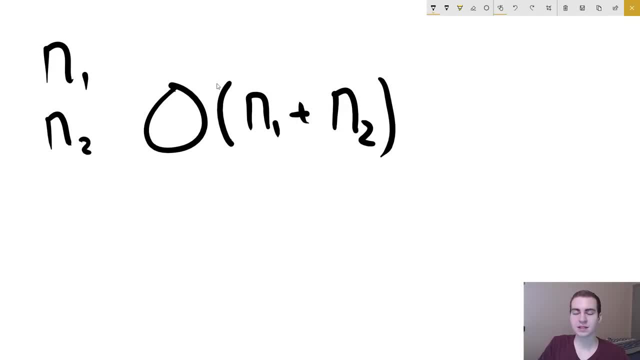 like way larger than the other one. So we need to keep both of these. So whenever you have kind of two variables, you have to keep them both, Alright. so now we've kind of talked about that a bit. we're going to show- I'm going to show some more advanced examples. 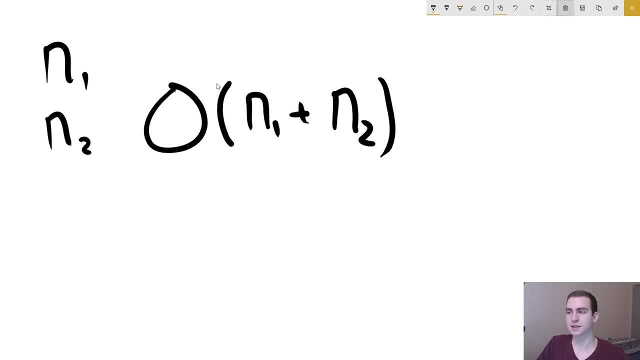 of like big one notations and how you kind of simplify them And then we'll actually start analyzing and hopefully it'll start making more sense. Okay, so now I'm just going to look at a more advanced example and how we can simplify this And remember we really 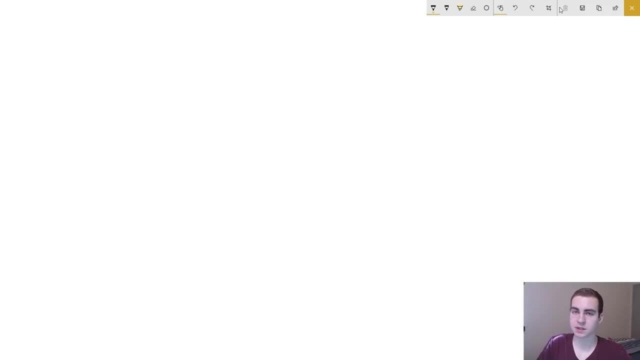 care about the shape of the function, right. So what we're going to do now is: this might be a bit complicated to you guys. you might not understand why I'm doing this, But I'm going to say, if we have a function that's like three n cubed. 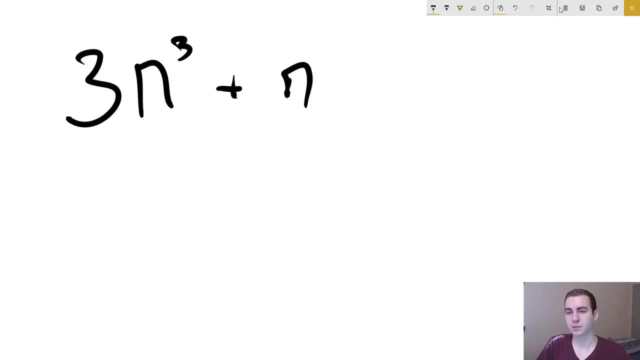 plus n. okay, How do we simplify this? Well, first of all you'll say, okay, we can get rid of the three. Correct, So now we have n cubed plus n. Now the thing is, what term in here defines the growth of the function which one increases the quickest? Well, n. 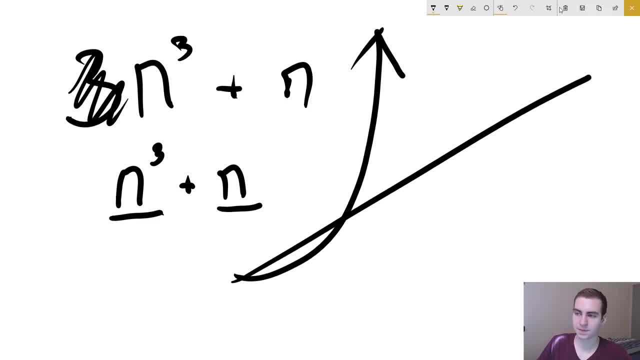 cube is like who like that, whereas n is just a straight line. So obviously n cubed is the faster term, So it's the more important term. it really dictates how large we the inputs going to get. like 1000 cubed is a large number and then you're going to add 1000 to it, right? 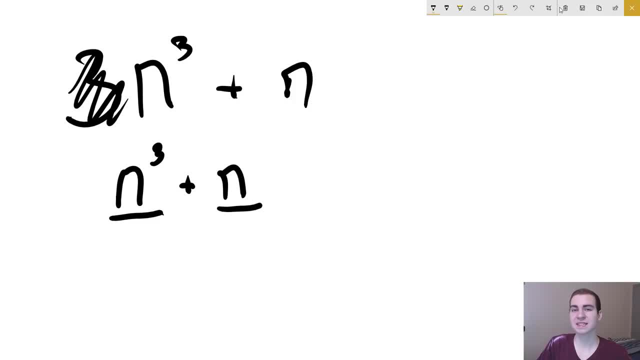 So what we can actually do here is we can simplify this to just be n cubed. Now why can we do that? Well, first of all, these are the same variable. Okay, that's important to know. if this was n cubed plus like n two, so n one cubed plus n two, we couldn't do. 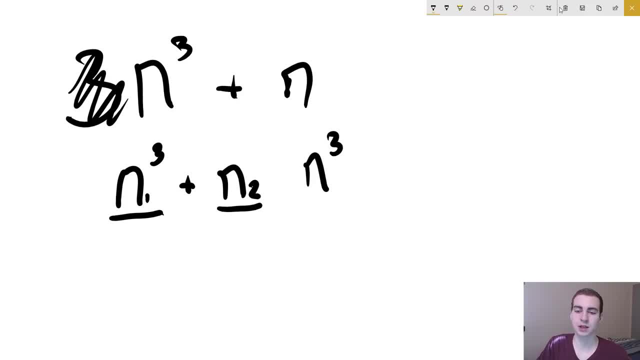 that, Because n two could be like a massive number which would actually change this right. So the different variables, we need both of them. But if we have the same variable, so n cubed plus n, n cubed really dictates how the function is going to grow. 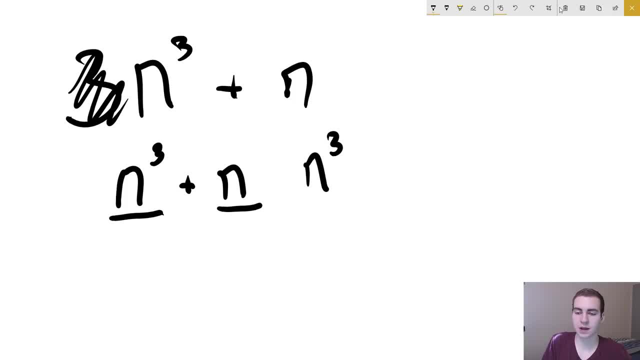 And that's the principal term, that's what they call it. So we can simplify this. So n cubed plus n to just be n cubed, And that's important. understand we're not going to. this is like a bit more advanced when you start doing stuff like this, But that's just important. 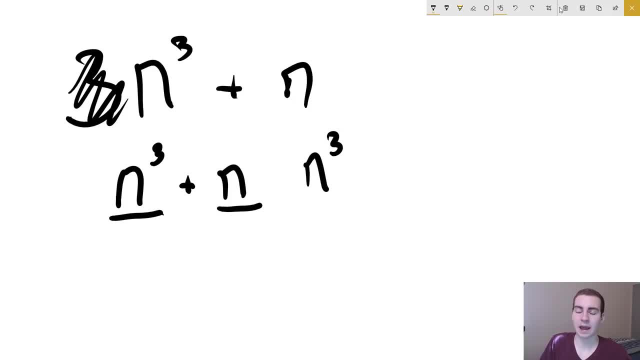 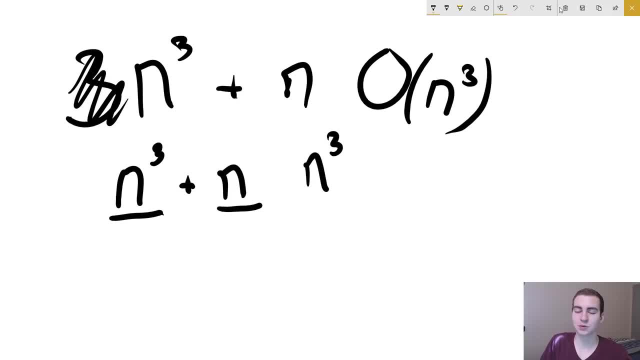 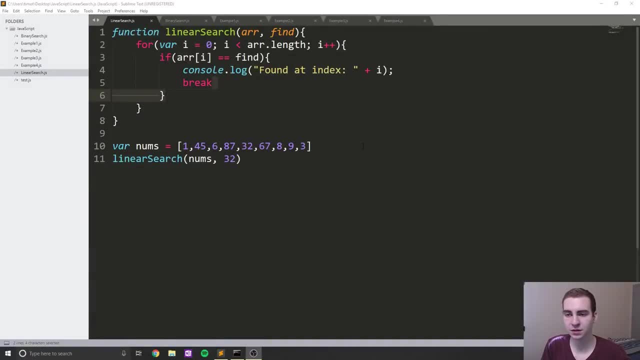 we're going to do this, And then we're going to do this, And then we're going to. actually, this is big O of n cubed, because that's what dictates how fast it grows. Okay, so now we're done with all the drawing. let's start getting into actually the real analysis. 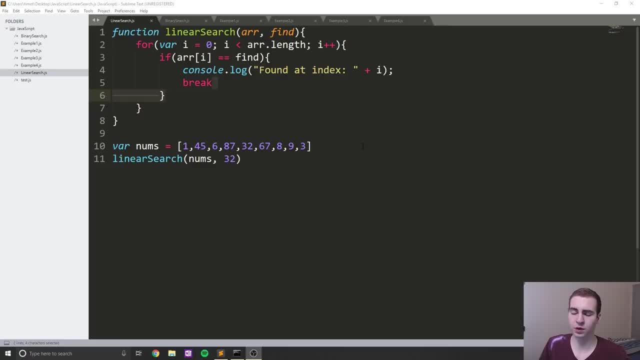 Actually, we're probably going to have to still draw, but I'll, like we're gonna read through some of these algorithms, which should hopefully be a bit more exciting and entertaining. Okay, so close that. So this is our first algorithm, And this is known as the linear. 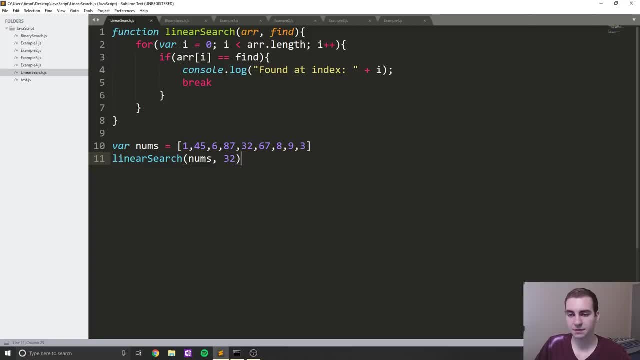 search algorithm And essentially what this algorithm does, is it given some input, so of size n in this case. we're giving it a list or an array. it's going to find a given number. So, for example, here we have this list or this array. sorry that has how many elements? 12345678910.. So we 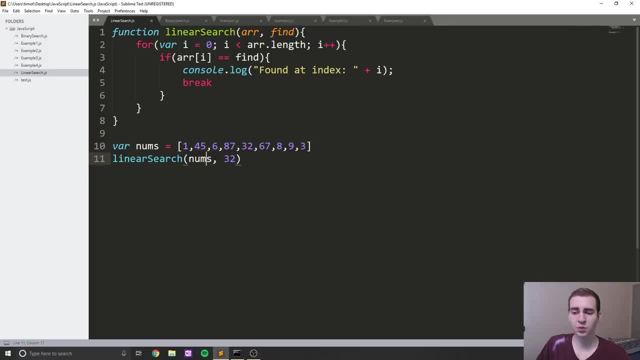 have n equals 10, right 10 elements, And then what we're doing is we're going to pass to our function the array and the number that we're looking for, And it's going to attempt to find this number, the index, where it occurs. So what this does, it does has a for loop And it looks. 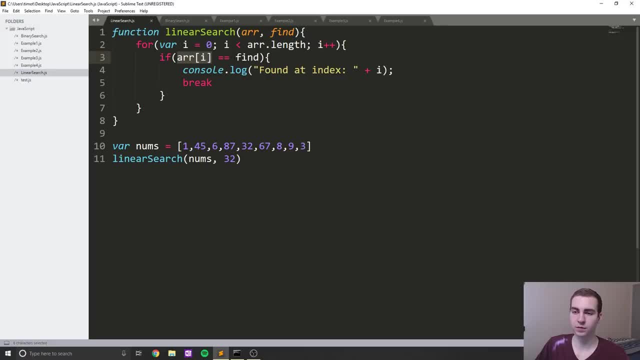 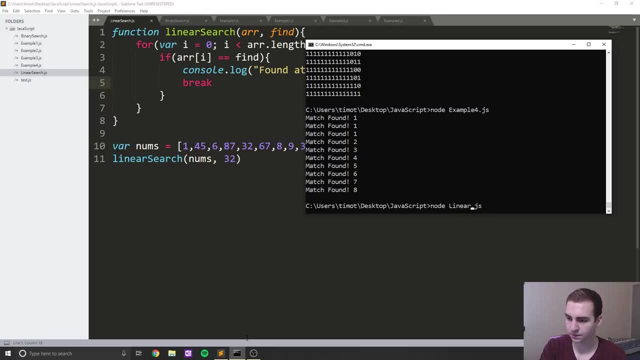 and it says: if we find a loop through the array, if we find it, we'll log that index. So let's just first run this. you can see I've been testing them here, So I'll just call this one Linear. 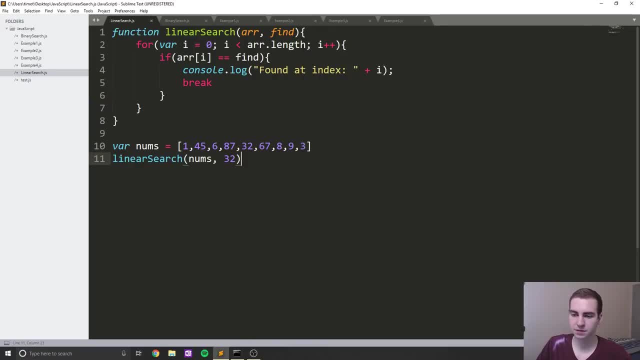 search, Okay, and you can see: found at index four. So essentially, it found 32 at index four, which would be the correct index for 32.. Alright, so how do we figure out the big O notation of this function? This is our algorithm, right, And we're just. we're using the algorithm down here, But this: 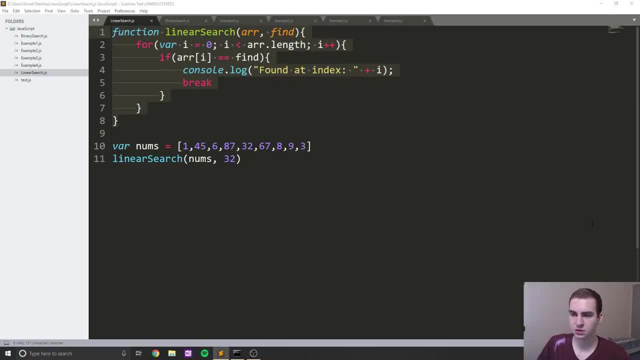 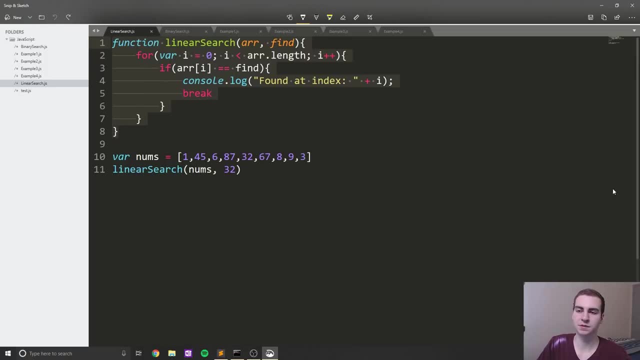 is our algorithm. How do we figure out the big O notation? Well, let's try. Okay, so this is our algorithm, obviously, the stuff that's highlighted. what we want to do is figure out how long this is going to take to run in terms of n. 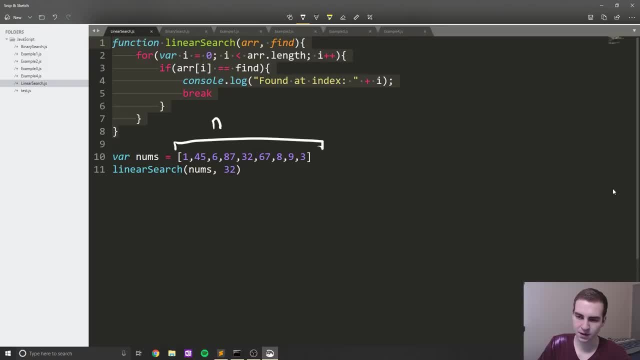 so ARR. So this right here is n. okay, And this can change. obviously we could have more elements, we could have less elements. So ARR up in this parameter is going to be length of n, right, That's what we're saying. So that's length of n. This list down here is what we're. 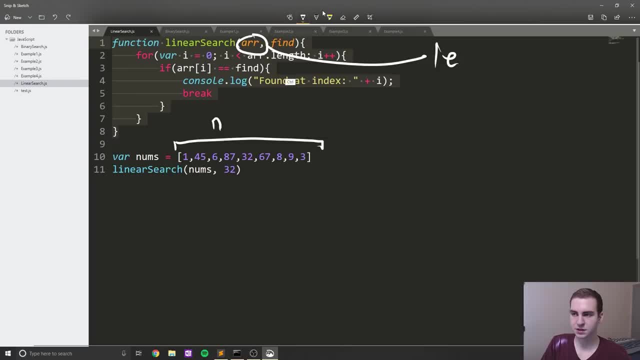 passing And what we're doing. let's actually let me undo all this So we can actually see everything that's happening here is. you see, we're going to loop through the entire array. So essentially we're going to say: I is going to go from zero, dot, dot, dot. two n minus one right. 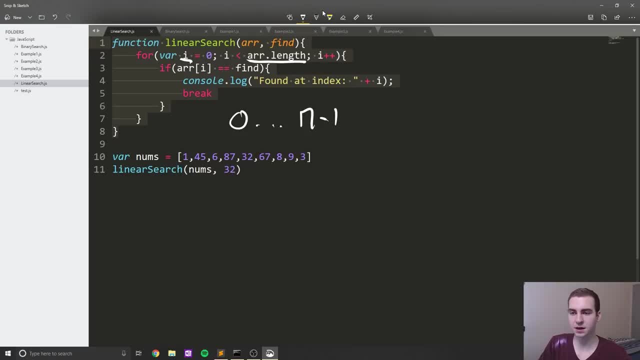 because we're going to loop through the entire race with the length is 10, will be only go to nine because index nine, hopefully, hopefully, you guys get that. So how many operations are we doing based on an input? n? Well, we're going to do all of this stuff n times. So what are we doing in? 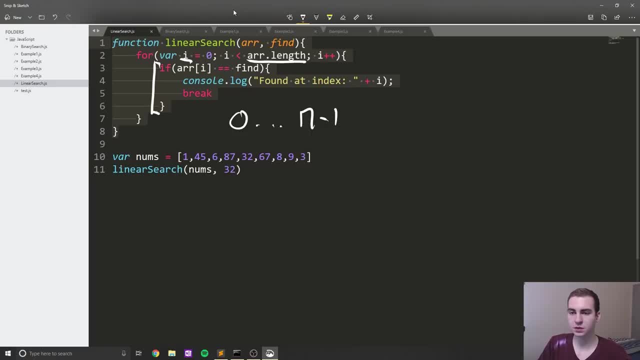 here right, Because it's gonna happen n times. Well, what we're going to do is we're going to log something And then we're possibly if we find that we're going to break, so we're going to end the loop. 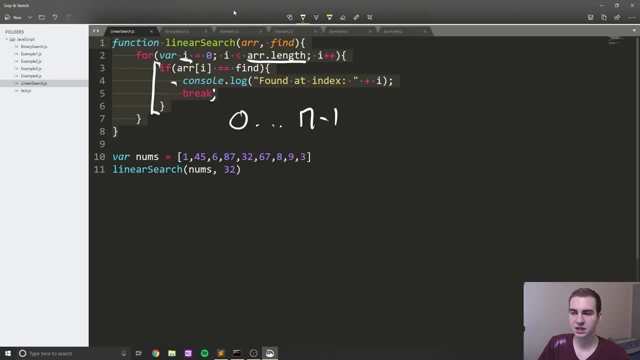 right, we're going to check something and then we're going to log something, So we could say that this is like one operation. because we're checking something. we can say this is two operations. you'd say this is three operations, But really right, like we're just doing one. 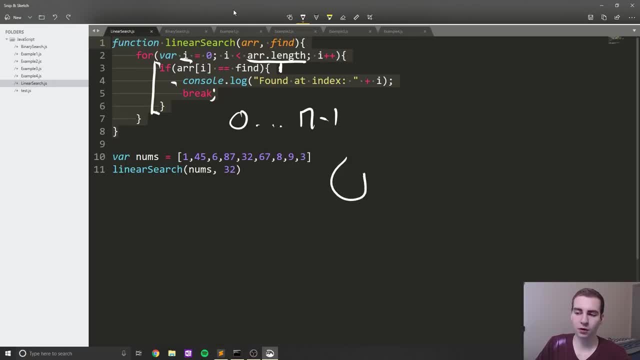 thing on each loop. So what we would say as well for our input n. we're going to do one thing each, So we're essentially we're gonna do n things. That's what we're going to do. we're gonna do n operations on our input n. So we'd say that our bigger notation is of n. 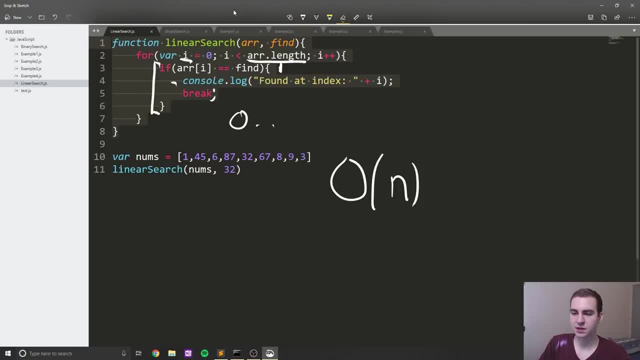 Now, some of you might realize, though, that we might not necessarily do an operations like: let's see if I erase all this right. So we're looping through the entire array, But notice that if we find the element that we're looking for, we're going to break, which means we're going to 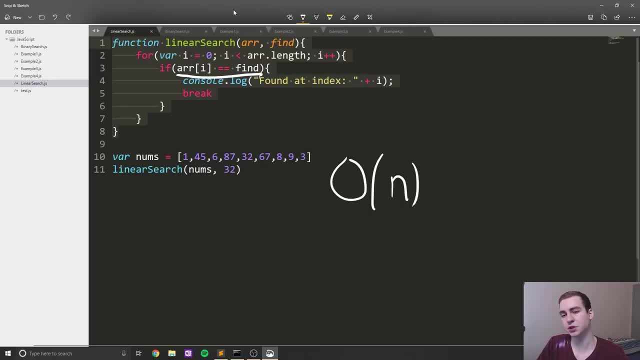 stop looping. Now, this is another important concept with bigger notation. So right now we loop, we go to four, right, So we're saying arr dot length, which is what? 10.. So we're going to do this 10 times, so n times. But if we happen to find the element before, 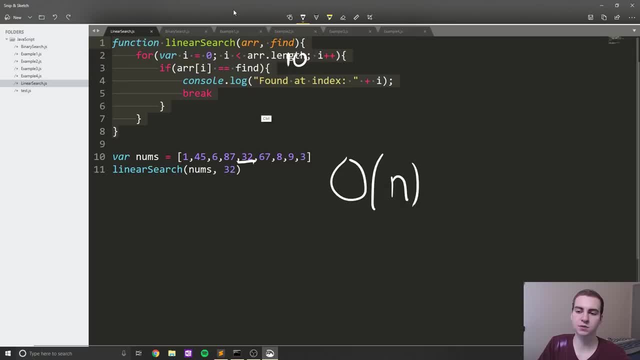 we reach the end of the loop, we're done, we're going to break out of it and we're not going to continue looping. So why wouldn't you say that this is big O of like a constant, like, let's say, 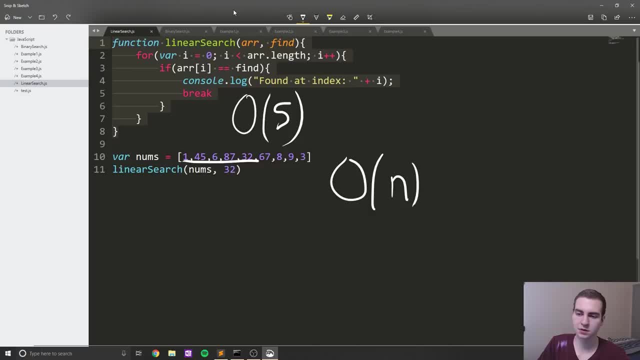 five, right, Because we only need to run that loop five times until we reach 32.. And we end. Well, the thing is, we don't know how many times we might have to loop. In a worst case, this element 32 could have been at the end of the list, right, And in that case it would have taken us well. 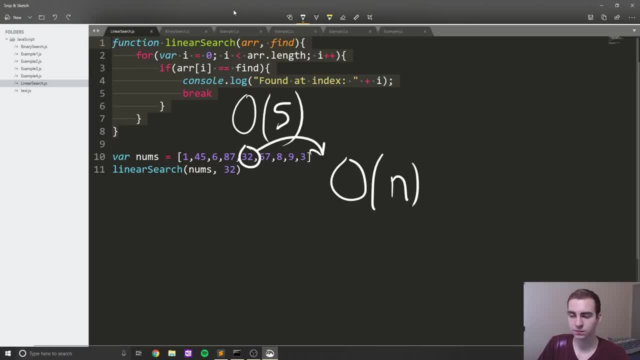 and the times and loops to find that element. So we're always looking at the worst case, which is what is the worst case that this algorithm runs in? So, for example, the worst case for this is that if we have a list where 32 is at the end, that would be the worst case for. 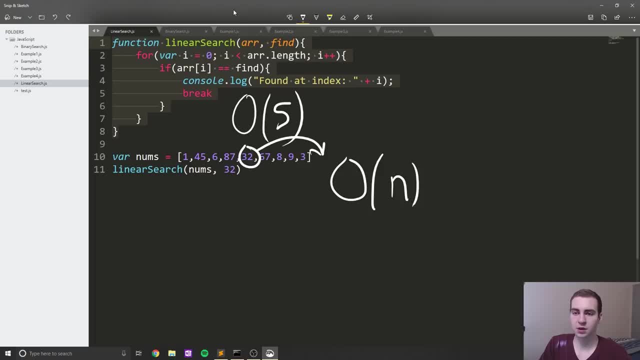 this algorithm, it would take longer. Why would it take longer? Well, because we're going to break once we find the element. But if we don't find the element until it's at the very last index, that means we had to look through the entire list. So we had to do n times, we had to loop n times. 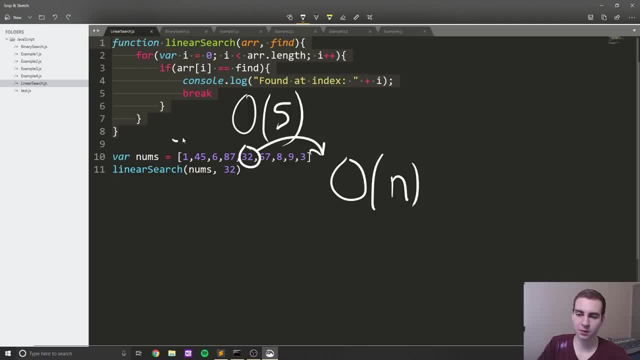 until we eventually found the element. Now, the best case would be if the element was at the beginning. So if we had 32, instead of one right here, then we would simply loop once: well, we'd say 32 equals 32.. And then we'd print it out, we would break, and that would only take one time. that'd. 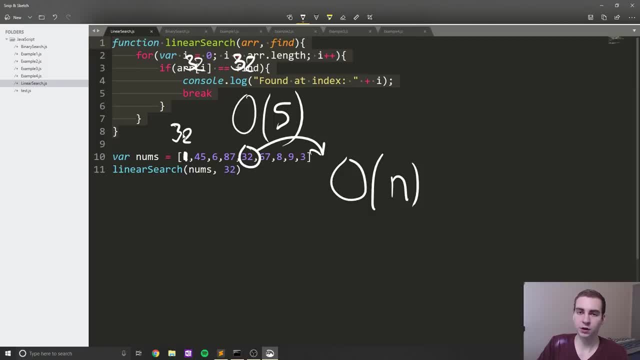 be one operation, But the thing is we don't know where our elements going to be, because this list could change. right, This list could be any size, it could have a different amount of elements. So we're always caring about the worst case, which is big O of n, because 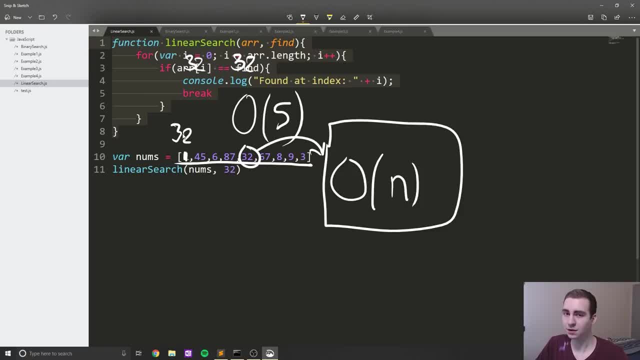 we could at most loop n times. So it's like it's unlikely that we'll loop n times. that'll be at the end, But it could happen. So we need to account for that And that's how we do this. It's always the worst case. you're never thinking about the best case you're. 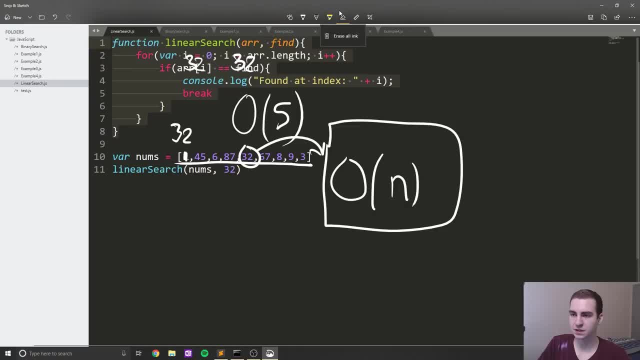 always thinking about the worst case. I wish there was like a clear for this, Because this eraser isn't really working. Well, okay, let's just close this, Alright, close, Okay. apparently it doesn't want to close, So give me a second, guys, I'll try to figure this out. 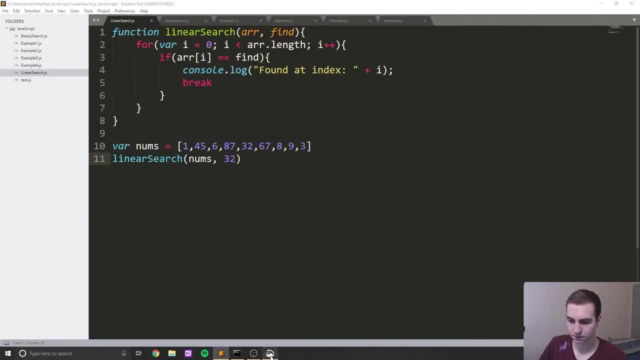 Okay, okay, Okay. so I got that closed. Anyways, so this is that's our first algorithm, And this runs in- we'll put a comment here- big O of n, which is also known as linear time. So essentially, 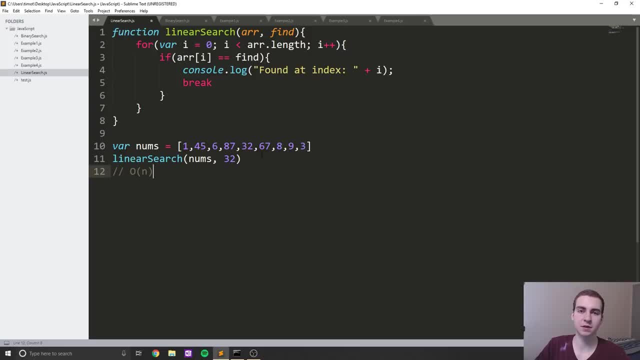 the longer the list gets, the longer it's going to take and it's linear, So like if the list increases by one, it's going to be at most one more operation we'd have to do. So this is big O of n. hopefully you guys understand this And we're looking at this. 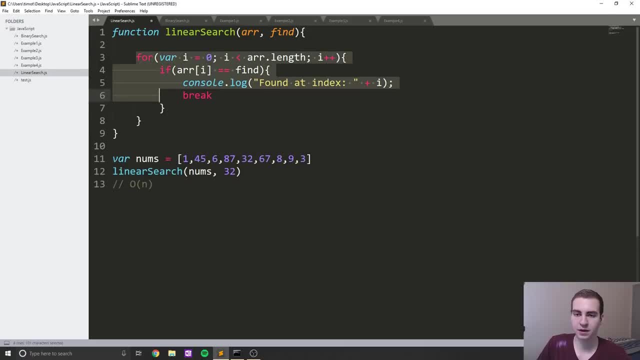 right, it's one for loop, which means that this loop could run at most n times inside the loop. we do a few things if we find the element, but we really only care about how many times the loop is going to run, because that's what's. 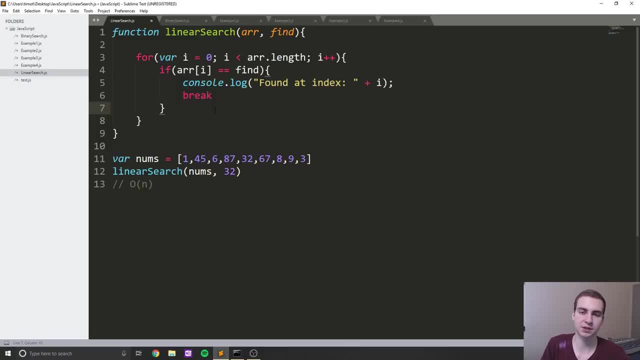 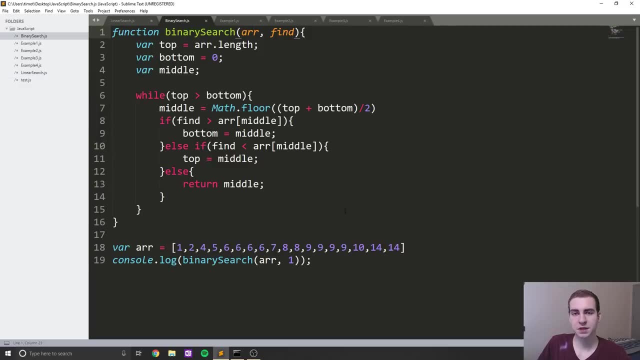 going to dictate how long it takes for this algorithm to actually execute. Okay, Alright, so next one. that was our first one: linear search, binary search. So you guys might have heard of this before, But essentially what this does is given a sorted list. it's going 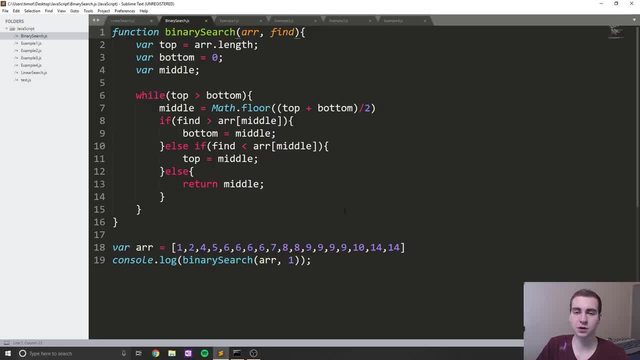 to find. it's gonna do the same thing as before: it's going to find the first occurrence of any element that we give it And it's gonna tell us where it is in the list. So let's just run this first of all. 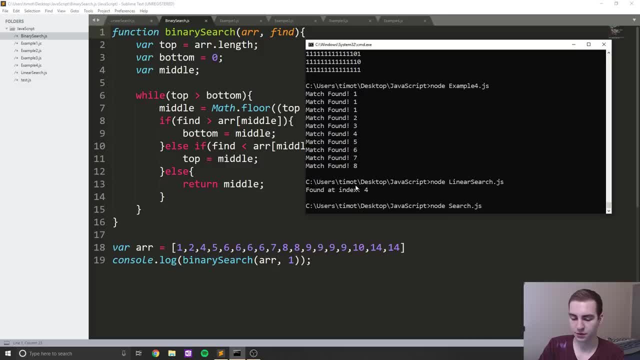 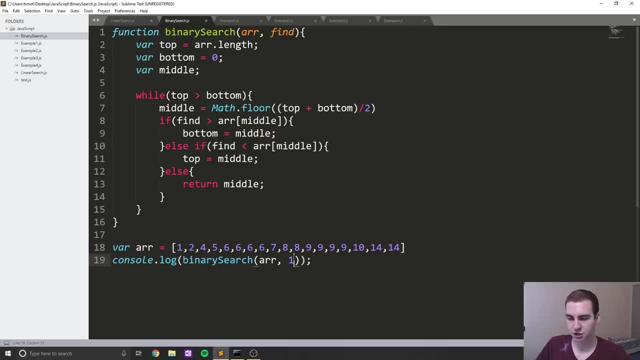 So I say, by the way, I'm just using node j s to run this stuff. I don't know if you guys care, But anyways, we'll do binary search j s And you can see we found what finds one at index zero. if I change it to be like eight, I should find one of these eights for us. 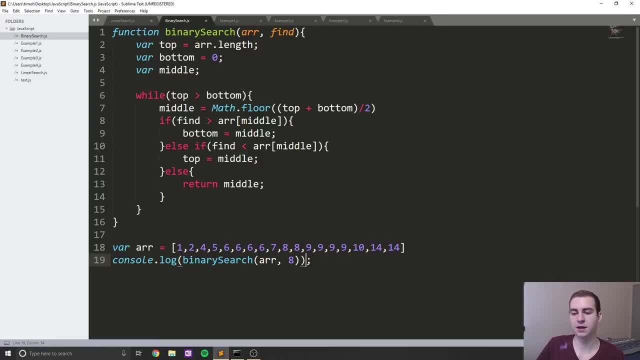 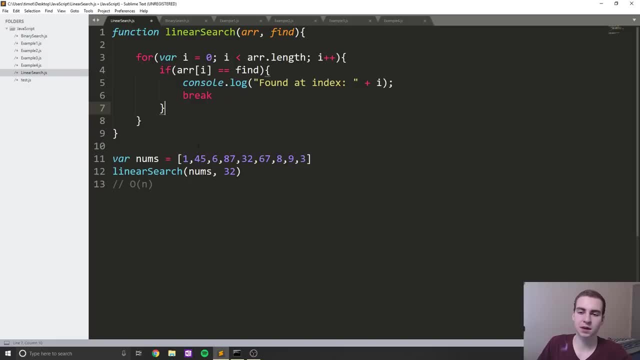 So let's run this And you see, it finds it at index nine. And I mean you can count the index if you don't believe me. So essentially it just finds the element. But the thing: why is this different than this? they do the same thing, right? 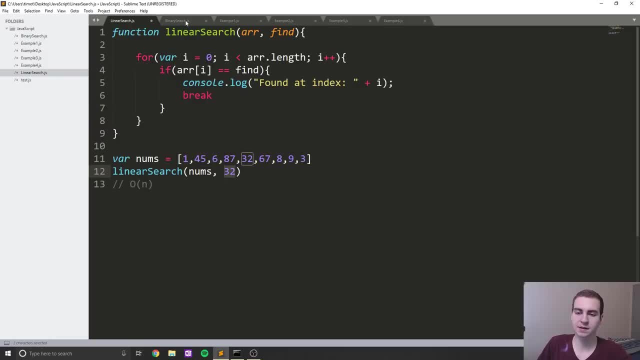 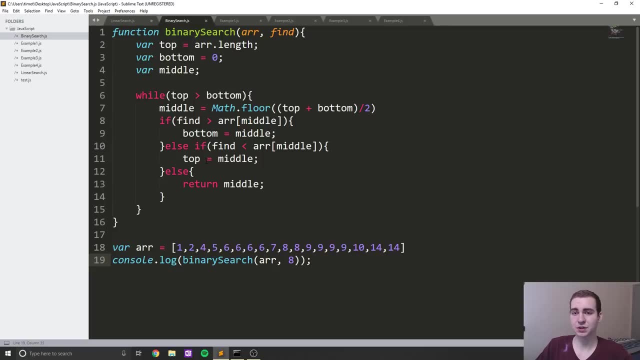 Given, given an array, and given a number, they tell us where that number appears. Why is this different? Well, this runs a lot faster than the last algorithm. And why does it run faster? Well, we're going to. we're going to talk about this right now And how this works. 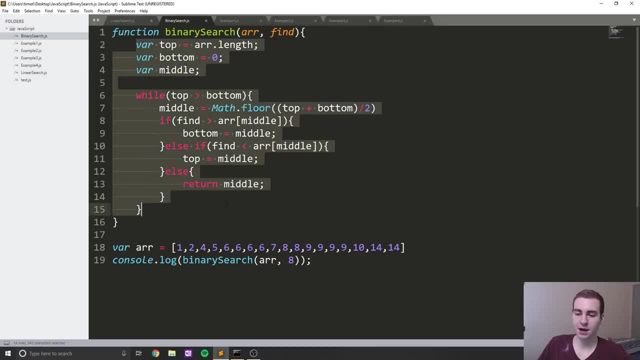 So this is known as the binary search algorithm, And why it's called binary is because it every time it runs, it decreases the size of our list, And you guys will see how this works in a second. So essentially what this does is it looks at. so we looks at the middle index of our 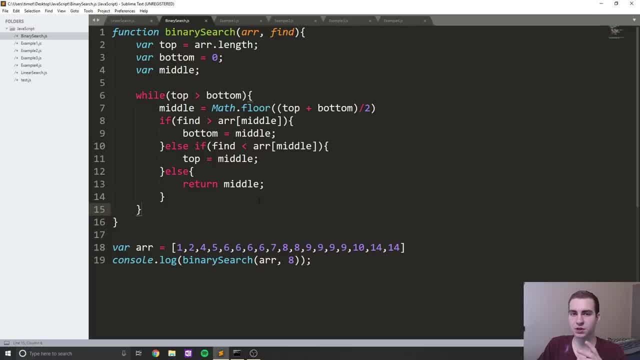 sorted list And think about if you have a sorted list and you're looking for some kind of element. So we're going to look at the middle index and we're going to determine if that middle index is greater than or less than the element. So in this case we're looking 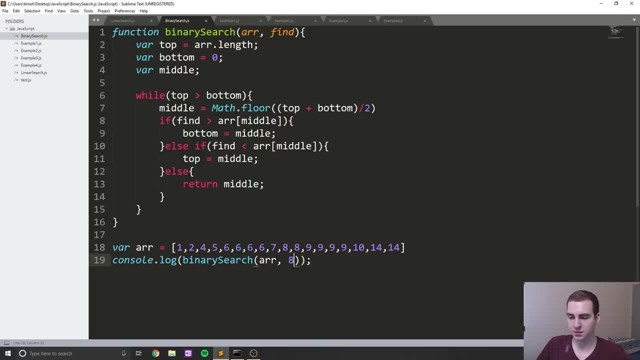 for eight. okay, the middle index in our list would actually be okay. let me change this to be like 10.. So it makes more sense. So we're looking for 10.. Okay, the middle index in our list would be something like eight. So we know this list is sorted, meaning it's. 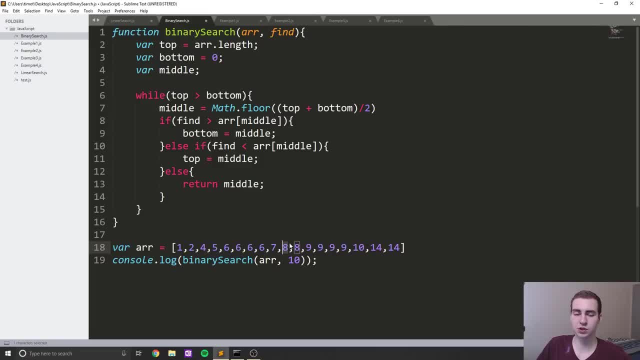 going from least to greatest. So if we look at the middle index, which is eight, we say, well, is 10 greater than or less than eight? well, 10 is greater than eight, which means that we know that 10 cannot. 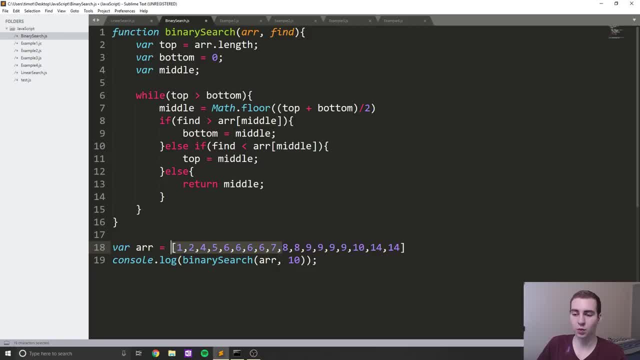 actually be in this left half of the list or the array. why can't it be there? Well, because it's sorted, And if eight is the middle and 10 is greater than eight, there's no way it can be behind eight. So why would we bother looking at any of these elements? Well, we. 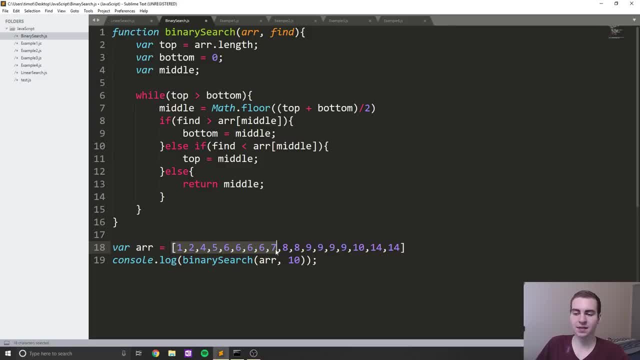 wouldn't and we're not going to, okay, so let's say we cut that portion of the list right. So the highlighted portion we're no longer looking in, And now we're. now what happens is our list turns into this, the highlighted. 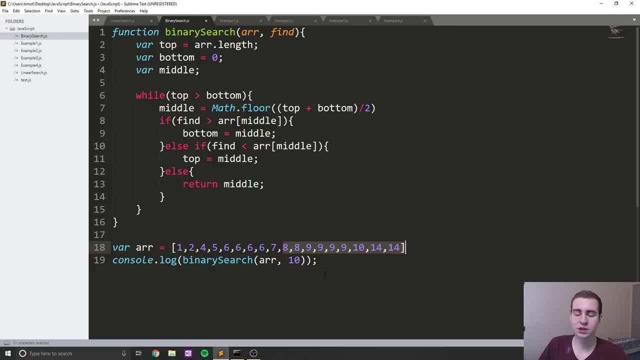 portion of 89999,, right, And we're still looking for 10.. So what we're going to do is now, our list is simply this, just this part with the brackets. So we're going to do the same thing we just did, Except with this list. we're going to find the middle index of this list. 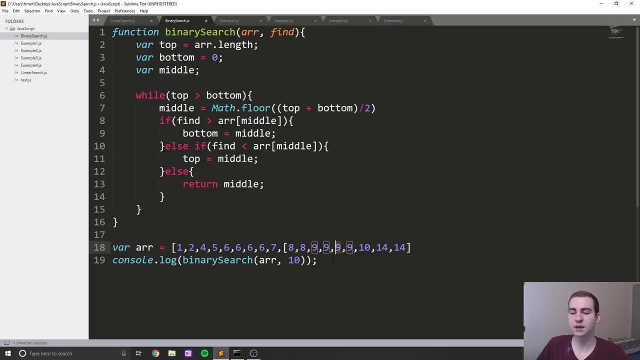 which in this case would be nine. And we're gonna say: is 10 greater than or less than nine? And again, 10 is the element we're looking for. we say, well, it's greater than nine, which means that all the elements to the left, 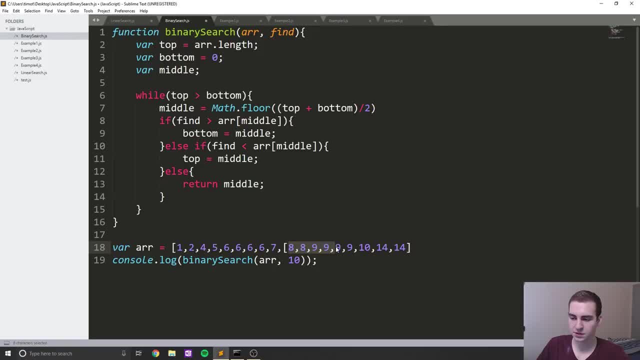 here are gone, we can remove them. So our new list becomes this: And now we say, well, why, Why would we bother looking at this portion when we know it can't be there right? So now we have this list, And now what we do is we look at the middle index, in this case. 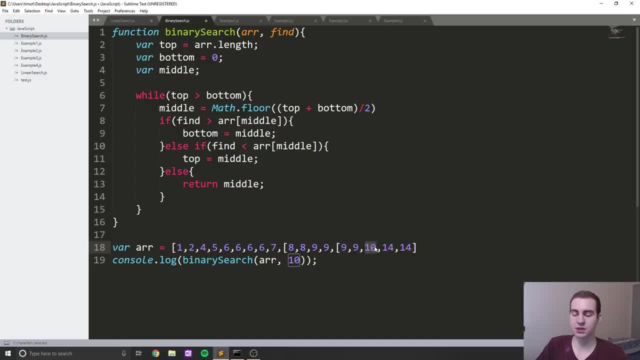 is 10.. And one of our checks is: is it greater than, is it less than or is it equal to? and we find that 10 is equal to 10.. We know what this index is and we return that to our- what do you call it? to our like from our function. So that's how the binary search algorithm. 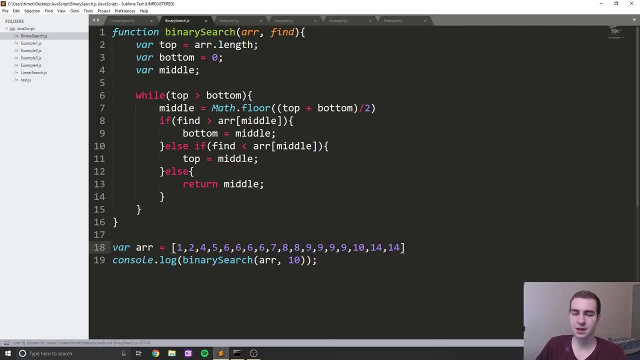 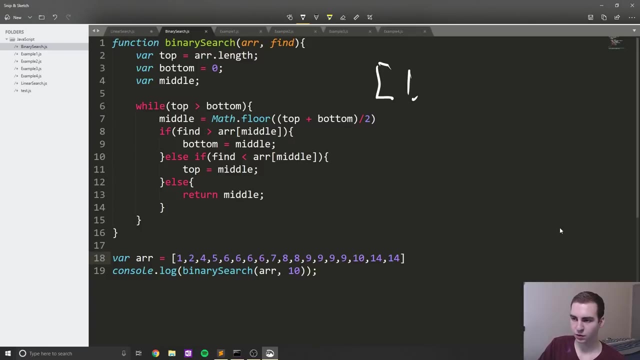 works. Now let's talk about how many operations this takes. So let's bring our up our drawing thing here, Or that's not the one I wanted. Sorry, one second. I want this one, And let's let's dissect this. Okay, right, So we have a list. Let's say we have a list of like 1234.. 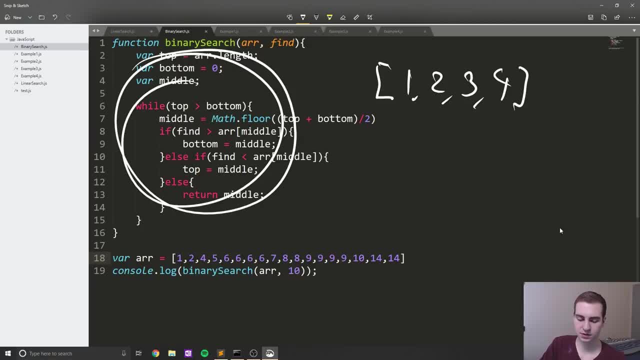 And every time we run this loop right, every time this runs, so the while loop here, which is right here, we split the list in half. So our first loop, we look something like this. our second loop looks something like this And our third loop would look like this: right, 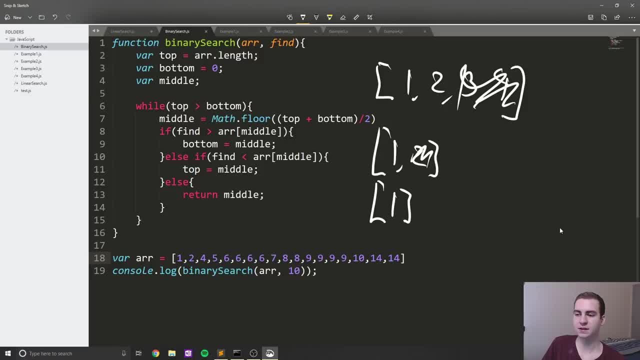 Because every time we essentially cut off half until we get down to one element, and the worst case for this algorithm is that we look through every single possible. what do you call it like? we look through the entire list until there's only one element left. 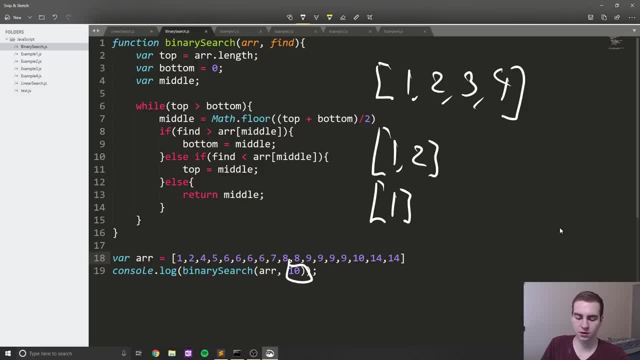 left, And then if there's one element left, it's either the element we're looking for or the element doesn't exist that we're trying to find. right, that's the worst case for this algorithm Because technically, like, say, we pick the middle index of two and 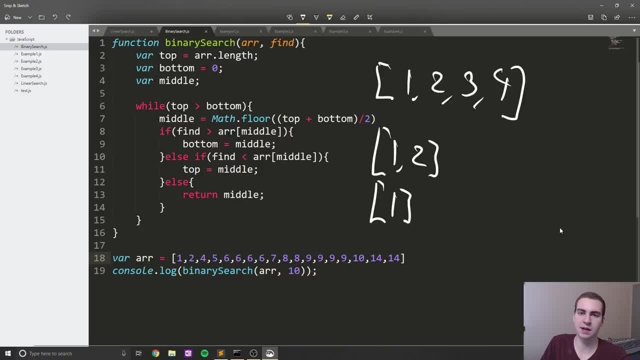 that's equal to what we're looking for. like, let's say we're looking for two, then we'll just return that index right away, So it could happen faster than possibly splitting it up all the way. Okay, so we split this up, split this up, and then we're left with this. So 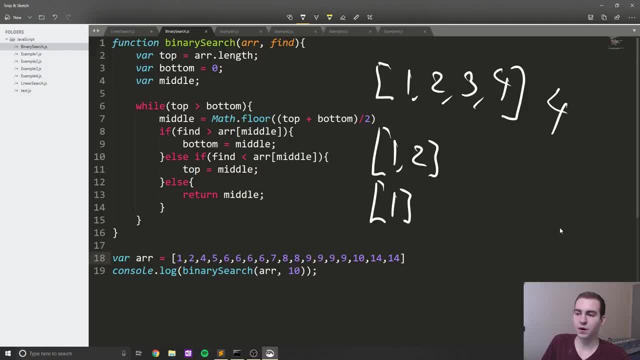 our input size was four, right, Okay, But we only ran at most three operations, really really only two, because this, like the first operation, brought us to this. we really only did two operations as operation one. this is operation two. right, we just ran the loop. 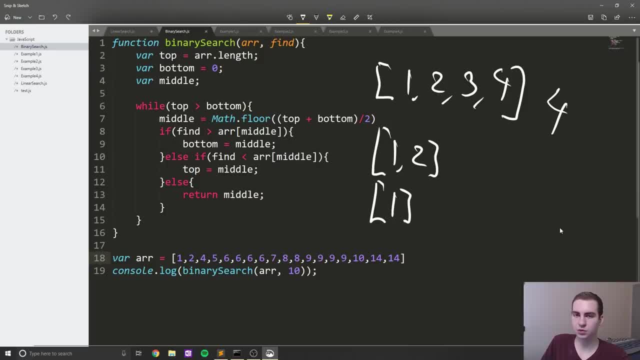 two times. we've ran two times, So what is that actually equal to? Well, I want you guys to figure it out, So I'm gonna do one more example. Okay, So let's increase this list now to be 5678.. Okay, so, now we've. 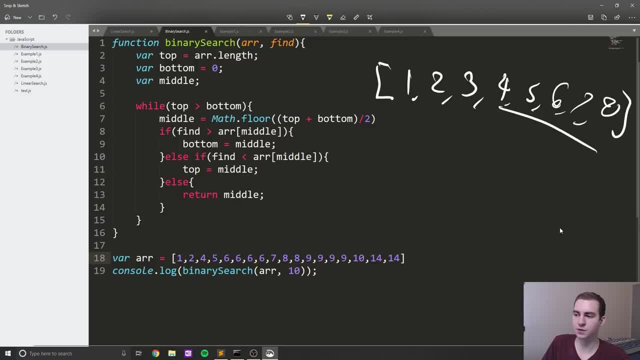 just doubled the size, So it was four, So it was to there. But now we've doubled the size and we've added those. What operations do we do now? So we start and we split the list in half. So we're either going to take the left side of the right side, So I mean 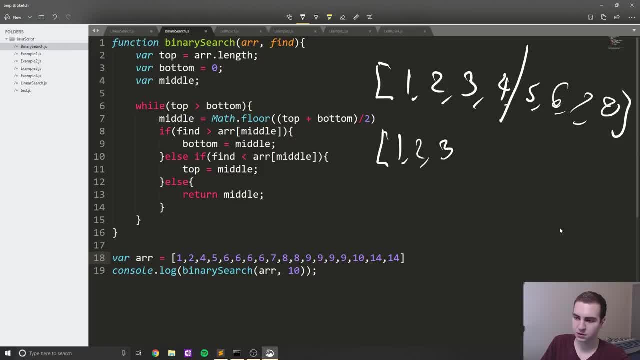 we can pick, it doesn't really matter, We'll say, we'll say we take the left side. So now we're at 1234.. Okay, now, what do we do? split this list in half. again one, two. what do we do? we split it. 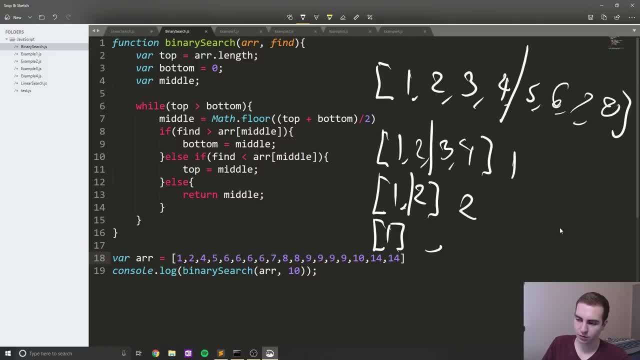 and we get one. So notice that now we have 123 operations. we doubled the size of our list and we only added one operation or one more run of this while loop, because this is what this while loop does essentially. But how does that work? Well, we're what function. 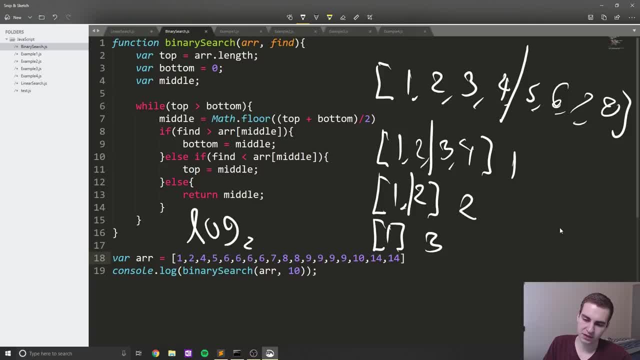 is this? we talked about it. this is actually log base two of n, And what that means is essentially is: based on whatever the size of our input is, we can find how many operations at most will run by doing log base two event, And log base two event is a function like. 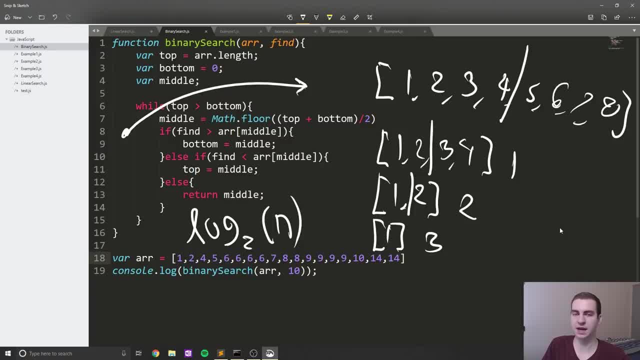 this that actually decreases in slope as it as n gets larger. So this is a super fast algorithm, right, And we would want to use this if we want to find something in a massive list. the only disadvantage of it is you need a sorted list, Otherwise you can't really. 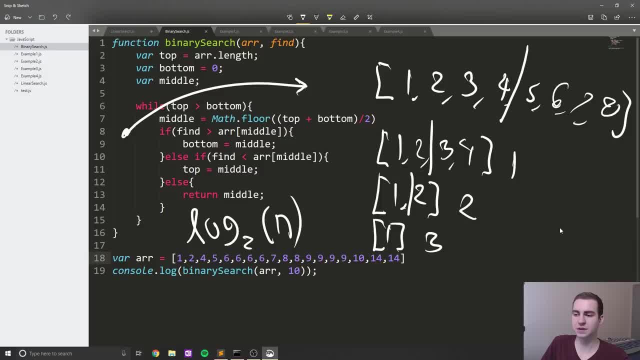 do something like this right If you don't have a sorted list, and that is essentially how it works In terms of binary search, and that's why it's log base two of n Now I want to talk about quickly. I really wish there was a clear thing for this man so I could Alright well. 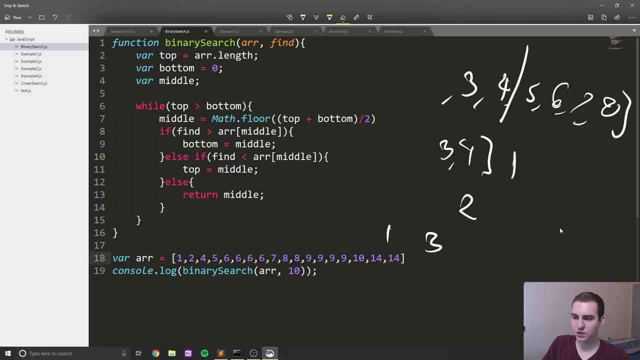 that's fine. It's flawed in the app. maybe I'll make one myself. But what we do here right is like: these are all the operations that could run each wallet right. So every time we loop through, like this wallet essentially is going to happen at most log log base two. 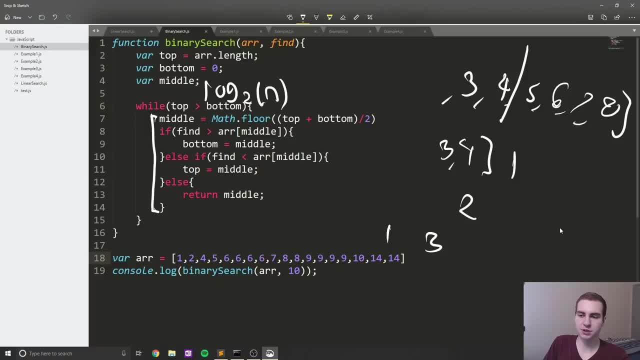 of n times. okay, But we do like a bunch of different operations in this wallet, Like, let's say we do this, let's just say we do like five operations every time it loops. Well, wouldn't you say that that's like five times log base two event. Well, you'd be correct. 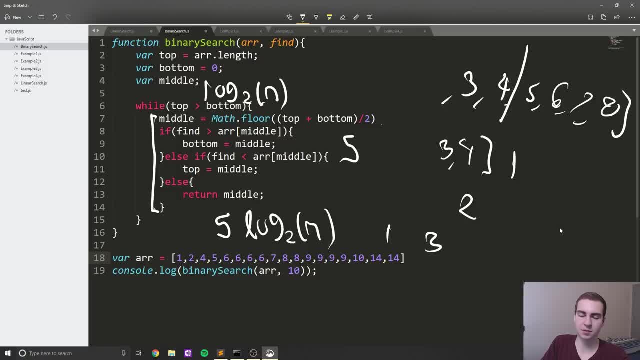 we do five operations. log base two times, right, Because this happens. log base two times or of n. sorry, But we do five operations. But the thing is, five is a constant right And we don't care about constants, So we just remove it And we say that this is then big. 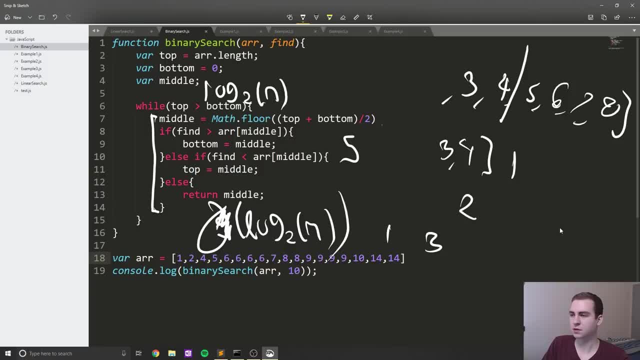 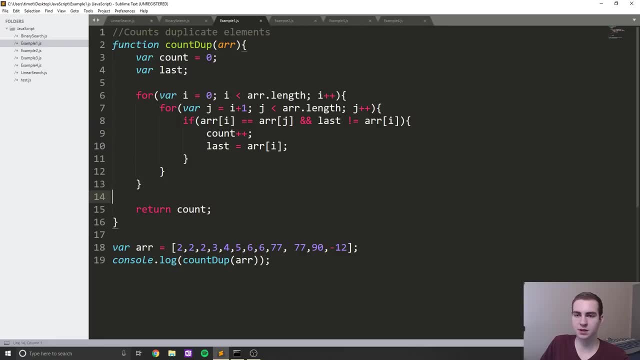 O of log base two event, And that's how that works. Okay, so we'll go a bit faster Now for these next ones. So now we're going to example one, and this one is just one that I wrote myself, And essentially what it does is it counts duplicate elements. So let's 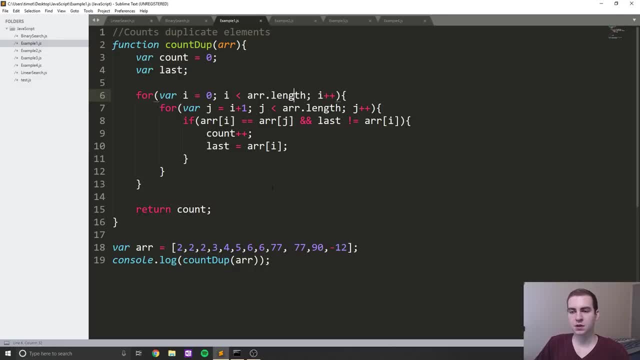 try to analyze this and figure out how long this is going to take. So the important thing to look at when you're analyzing something is the amount of loops right, Because, remember, we don't care about the constants, So all the stuff inside of these loops it doesn't. 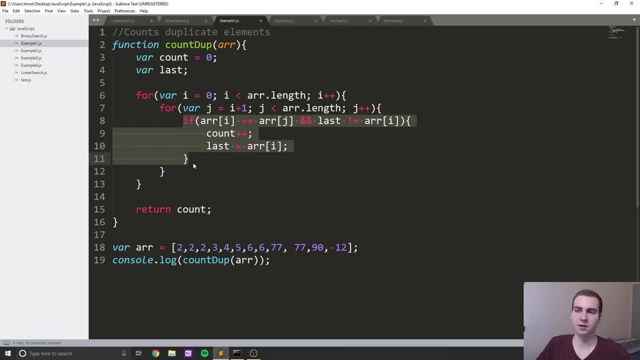 matter how much you're really doing, because we're just going to omit the constants anyways. like, say, you're doing something like n times, but you do like every n. you do five things, that's five n well, you just get rid of the five, So we don't care about. 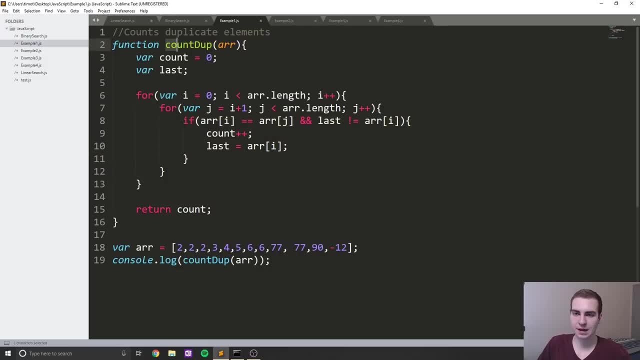 the constants, right. So how many times does this happen? we're going to count the duplicate elements. So essentially, given some kind of array, we're going to find how many elements appear more than once. So, for example, the like this one: there's two duplicate elements. 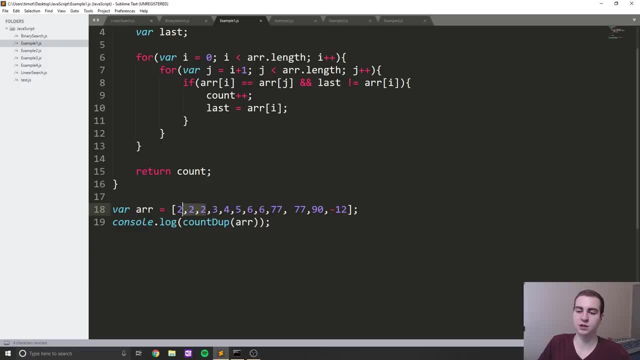 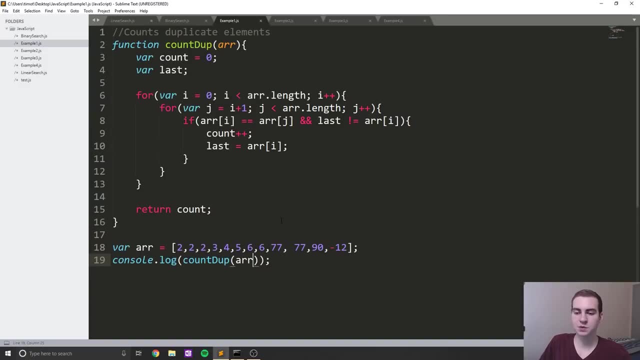 because two is duplicate and six is duplicate, Even though there's like three twos, just because two appears more than once, like that counts as once. you know what I mean? Like that it's a duplicate element, That's what we count. So I mean, I'll show you that this works first. 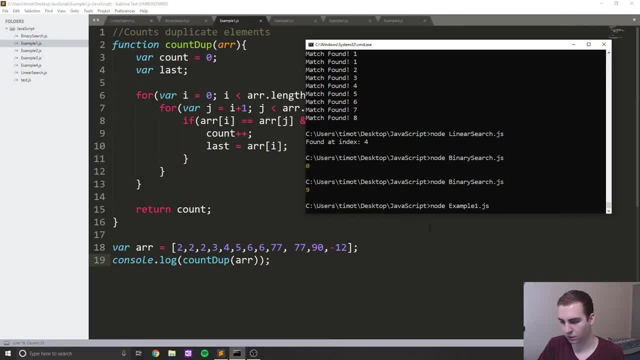 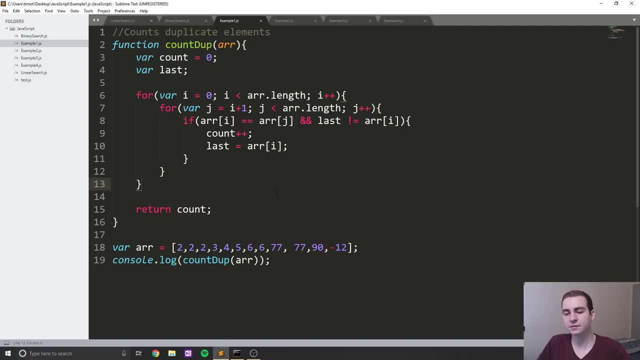 didn't mean to close all that. Example one. okay, and you see that we get three duplicate elements, And that's because 776 and 222.. Right, So how long, how many? How long does this take to run? Well, let's look at it. 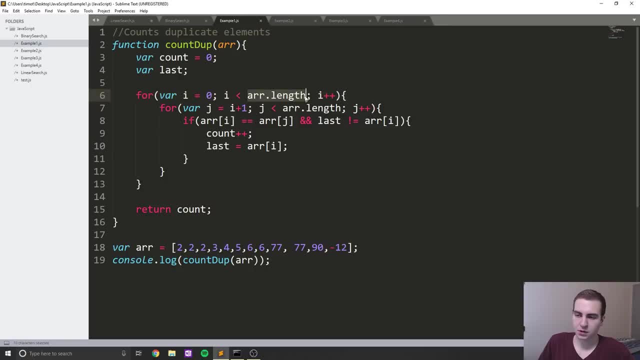 So what we're doing is we're looping through the array dot length. okay, So that's going to happen. what n times? right, Because array the length of our arrays and that's our input size. this is length and whatever that length is. so this is going to happen n times this. 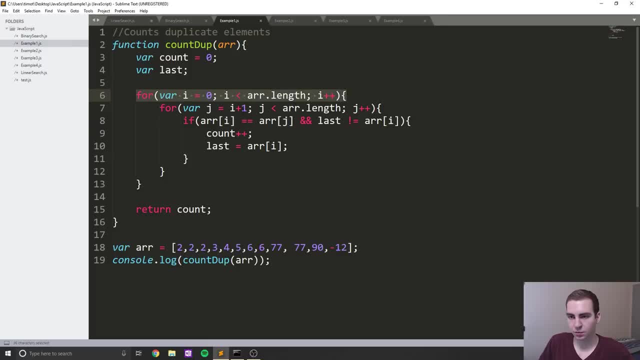 first for loop, But then inside of that for loop, what do we do? we loop again and we say we're gonna loop again through the entire list. So we're looping once, And then, every time we loop once, we're looping through the entire list again. 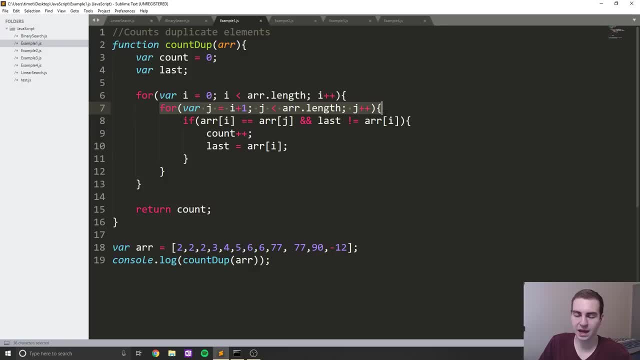 so essentially every one of these four loops we're looping n times. So every time that this runs, we loop n times again. So this run, this runs n times, but this runs n times And this runs every time that this runs. So we say that this runs n times like that, And 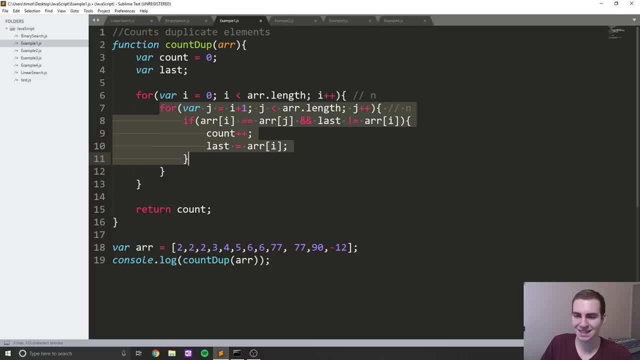 this runs n times, But since this for loop is inside of the other one, it means that every time that this runs, this is going to run. So you might be seeing what I'm getting at here. How, what it like, how long does this take to run? Well, this actually runs. 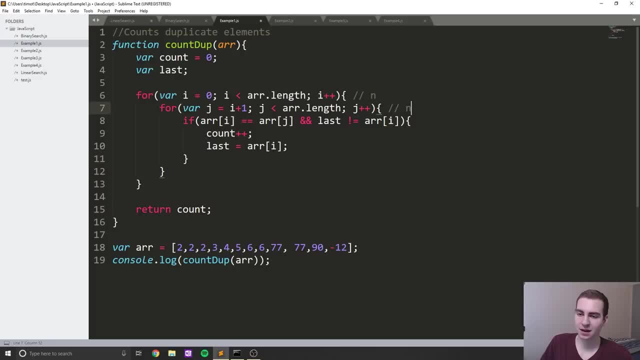 an n squared. And why does that happen? Well, because for every n we do something n times. So essentially that's n multiplied by n and n by n is n squared. So this is quadratic And as the length of our input increases, this is going to take a lot longer to run. 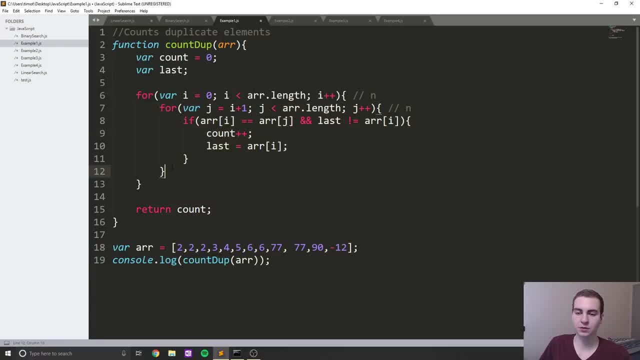 These are things we want to avoid is embedded for loops and embedded while loops, because, well, it takes a really long time to run, And if I were to put another for loop in here like this and say it does something, well then this would run, if it ran n times, right. 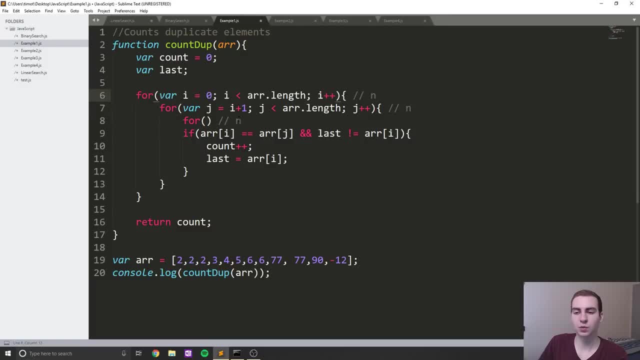 So this runs n times. this runs n times. this runs n times. So we're gonna run n cubed times, which is a crazy amount of times to be running right, So that's how we kind of do that. So I 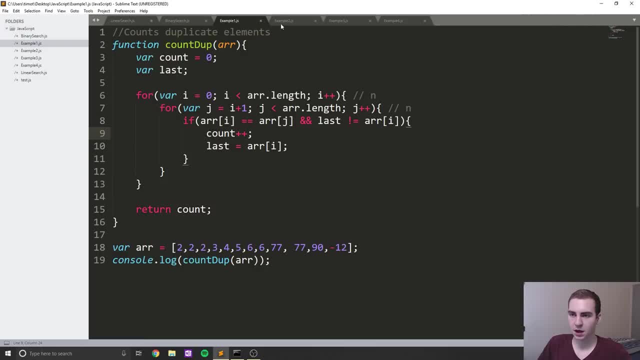 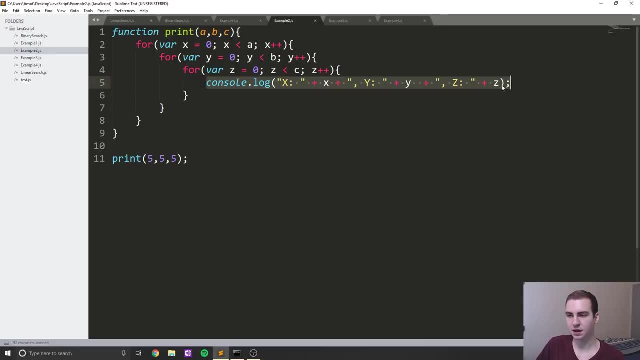 think that's, I mean, that one's pretty straightforward. I don't need to really do too much for that. Okay, so let's go to example two. example two: Okay, so all this one is doing- and it's really it's similar to last one- is we're just going to print x, y, z, And this is a. 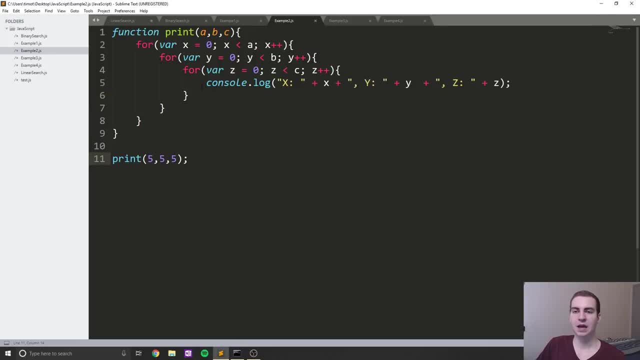 good example- Actually, I don't want to print it yet, it's going to give it away, But we do- is we take three variables like ABC, as our input, And what we're gonna do is we're gonna loop a times, B times and C times- okay, ABC times. So this one's a bit more. 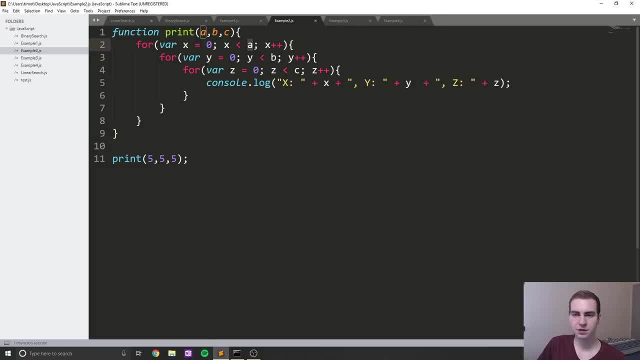 complicated, actually, how? What's the big O notation of this? How long does this take to run Right, So we can say A, B and C is like our n, like our input, how long it's going to take to run Well. 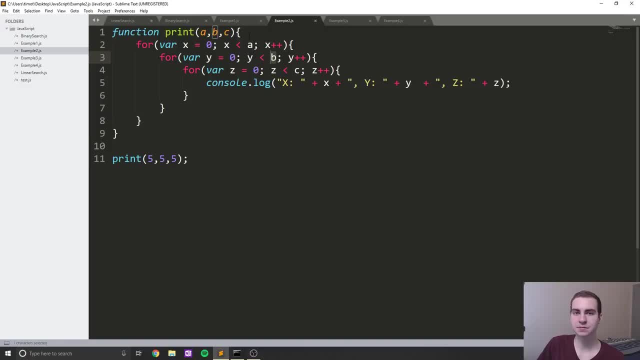 what we do is we run a times, we run B times a times. I know it's confusing, but we run this for loop B times every a time. So that's a times B, right? So we run these two for loops a times, B times. Now what about this third one? there's another for loop inside. 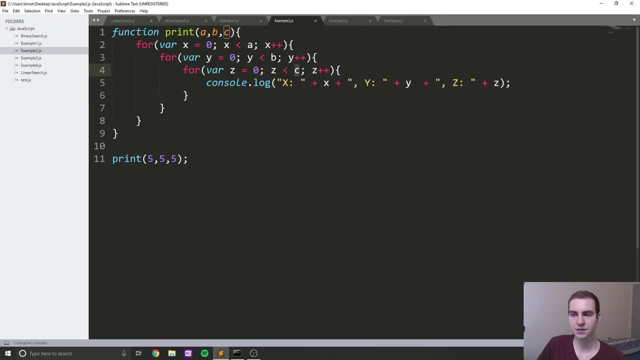 of another for loop. So this runs C times. So every time B runs this runs C times. And every time B runs this, every time a runs this runs B times. So this is actually a times B times C. Now what can? 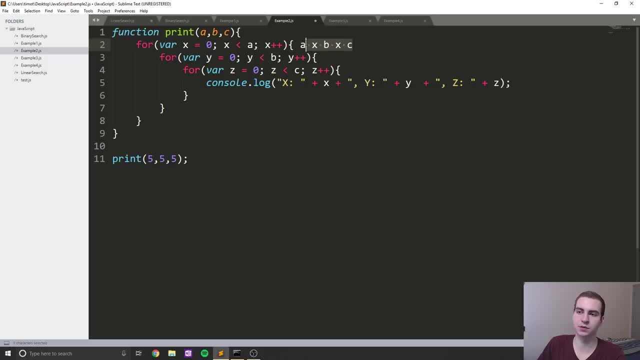 we simplify it to be like n cubed. Well, you can't, because there are three different variables. right? If it was one variable and it was like a, then we would say a cubed because it's a times a times a. But since it's three different variables, we say: this runs in a. 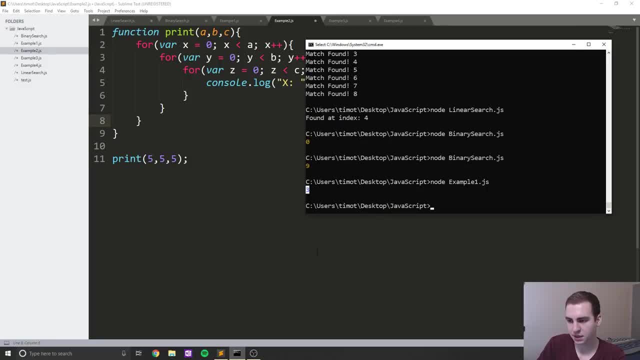 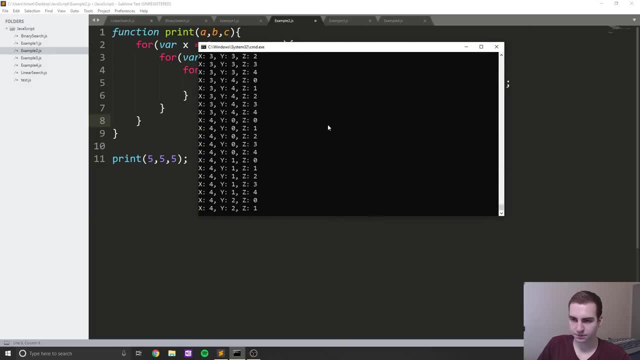 times B, times C, And I'll prove it to you. So I'm going to run this now. Example two: dot j s and watch my, watch my screen. Okay, So we get a bunch of output. Let's scroll through it. So this little lot, these lines of code, ran like this many times. 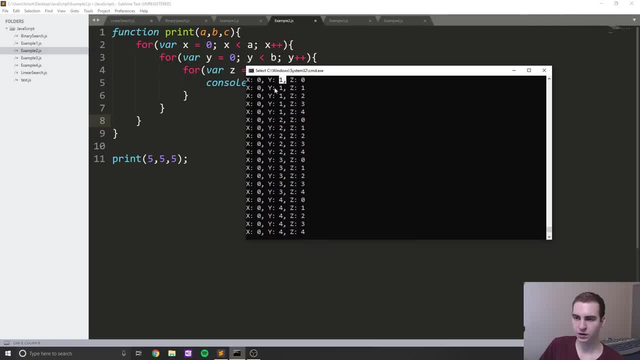 and you'll see. so we have: x starts at zero, y is one, x is zero, y is one, z is one, x is zero, y is one, z is two, x is zero, y is one, z is three. So you see that essentially. 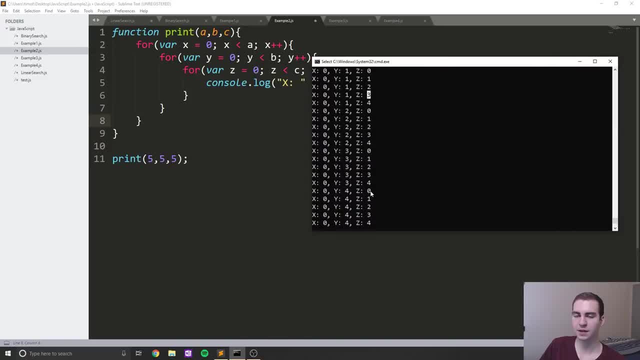 zed goes 1234, 01234, 01234.. And that runs a ton of times, Whereas x stays at zero and goes to one, goes to two, goes to three and then, once it's done, it's done. So you can. this kind of gives you an idea of exactly how this works, right. 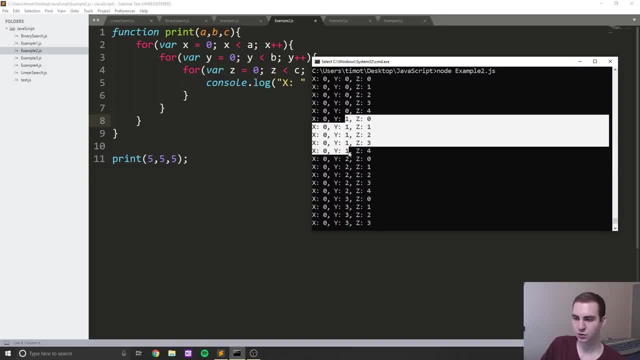 So you go x, zero, y, zero, 00, right, and then y will change to one, and then zed will change right, And that's exactly how it works. So that's how we can kind of determine that this runs a times, B times, C times. And I mean, if you want it to count these amount of inputs, 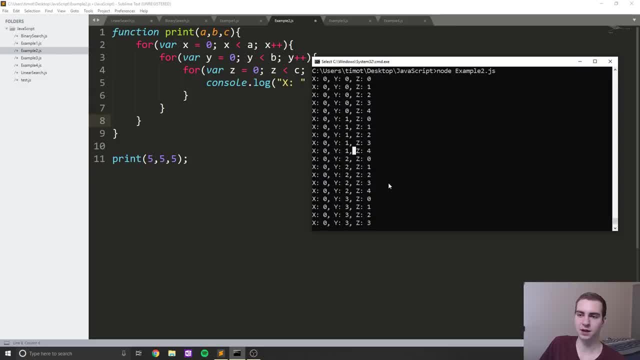 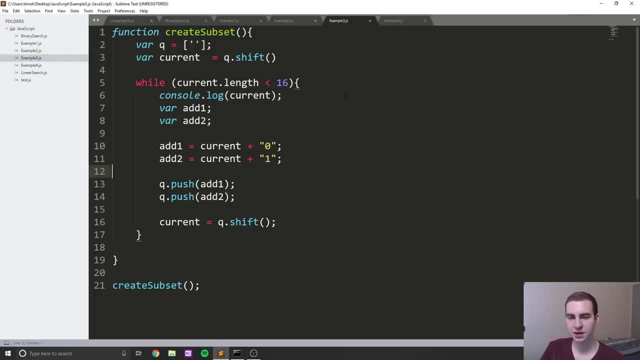 you would get five times five times five, which is essentially 125 lines. Okay, that's how long that runs. I don't want to close that. Okay, example three: So this one, okay, so this one actually is going to generate all. 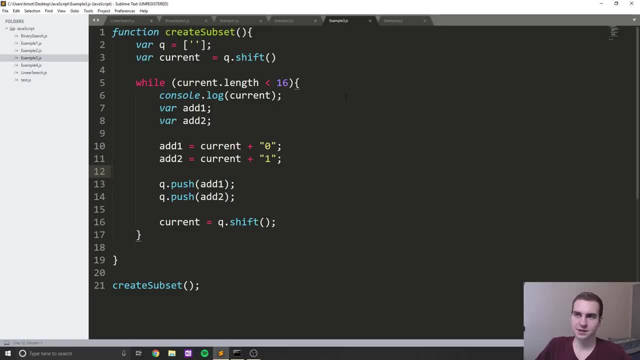 of the binary numbers from that are of length 16.. So it's going to start from zero and go to length 16.. So all of the binary numbers that are of length zero to length 16.. Does anyone know how many numbers that is? It's a lot of numbers. I'll tell you that right. 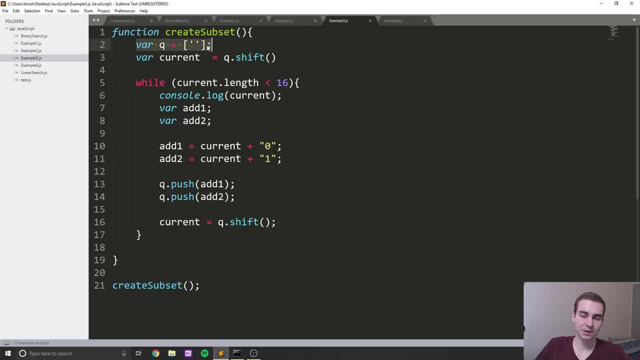 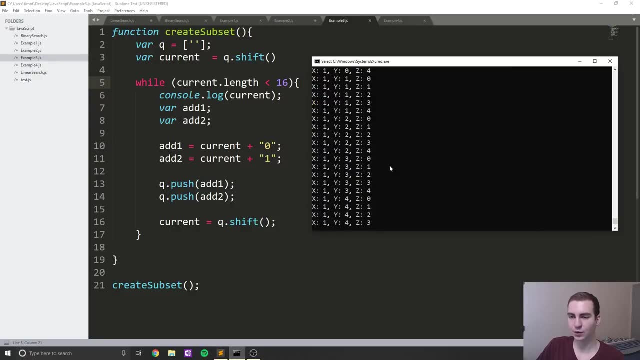 now. Now this works using something called a cube based algorithm. I'm not going to explain what that is because it's a bit confusing, But essentially I'll run the program And then let's try to figure out how long this runs. And okay, so let's go down here. It's example three: dot j s All. 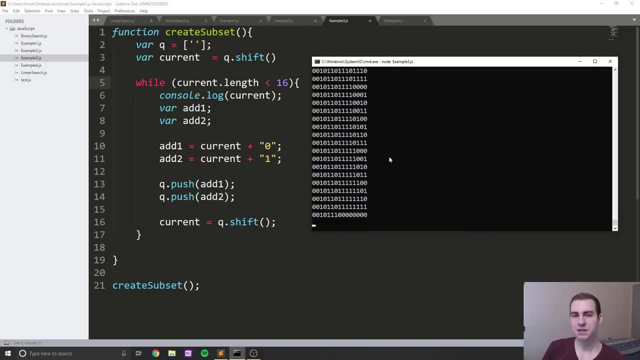 right ready, I'm gonna run this. Watch my screen. this is going to take a second to happen, And this is what I'm talking about with the time complexity right. I'm only making all of the binary numbers that are of length 16.. But look how long this is taking. 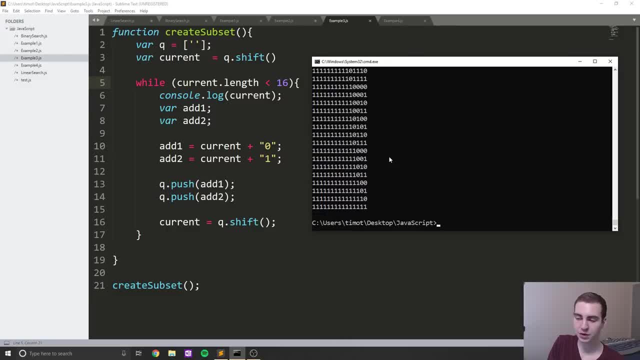 to run, And if we didn't know anything about time complexity and we weren't printing this out to the screen, we would not probably have realized how long this algorithm that I created takes. it's super inefficient, But it's really the only way to generate. 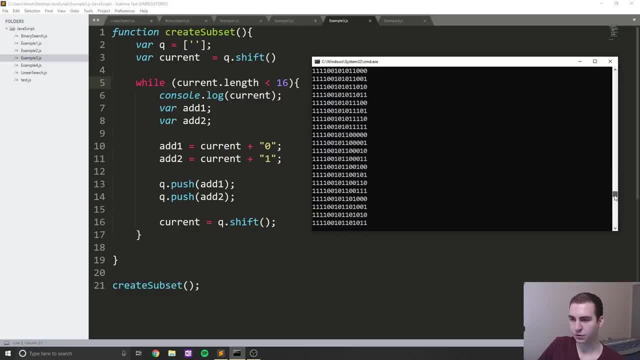 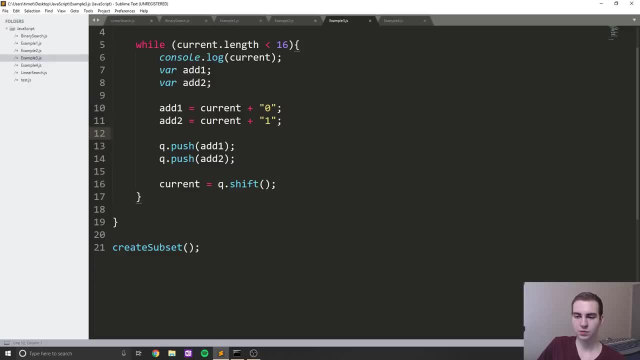 all of these different numbers So you can see. I mean, if you like, if you scroll through, we have a ton of different binary numbers. I can't even reach the end. the last input, like the start one, So this: how long does this take to run? Well, this actually takes. 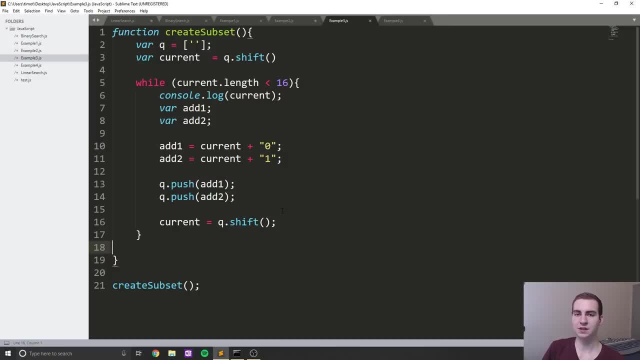 two to the n to the n times, where n is essentially like the length of the binary number which is going to be 16.. In this case- okay, because that's how many possibilities of binary numbers there are- two to the 16. And I mean we can prove that pretty straightforward. I'll draw 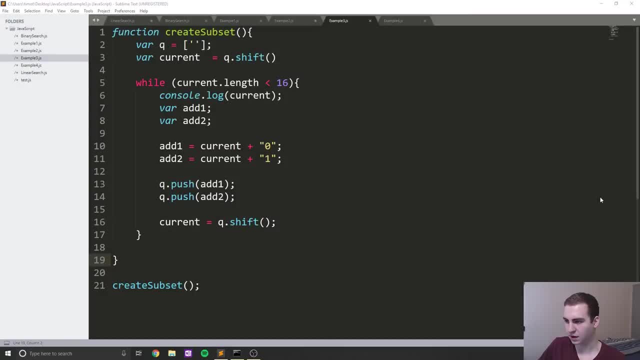 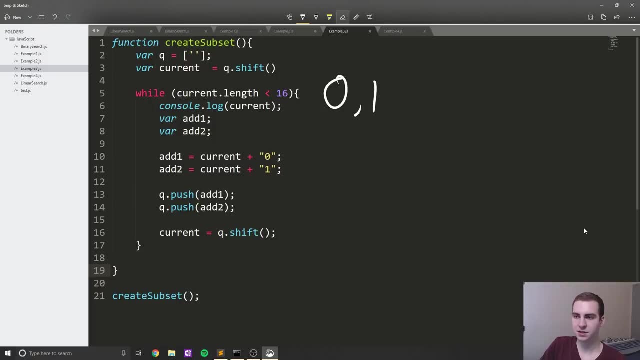 this to you. If you guys know anything about binary, don't want to use that, I want to use this, right. So, binary numbers: you can either be zero or you can be one. it's one or two And they can obviously have like an infinite length. So we're doing all the binary numbers. 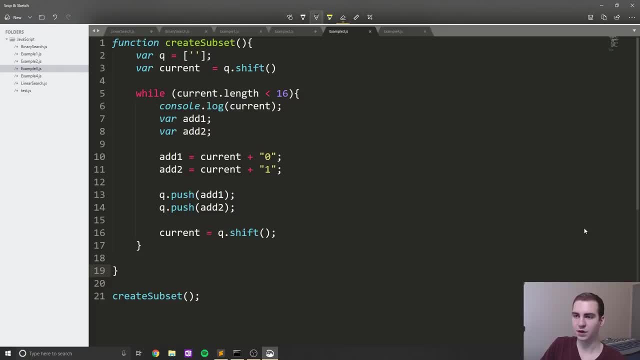 of length 16. Which means that we can- well, I'm not going to draw them all up, But let's do an example with three. So if we have three digits for a binary number, then we have. we can have 000, 001,, 010, 011, zero, and then this: sorry, this goes 100111.. No 101.. Sorry. 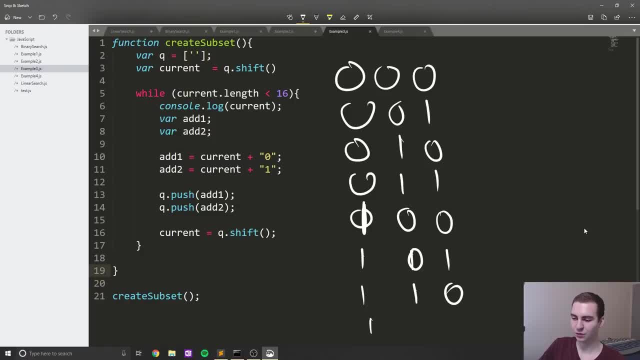 Why is this so difficult to do? One, one zero and then 111.. So we have 12345678 different binary numbers for three digits. Okay, for two digits, like let's just scrap. What row should we scrap? I'm trying to? okay, let's scrap this row, All right, And then have a. 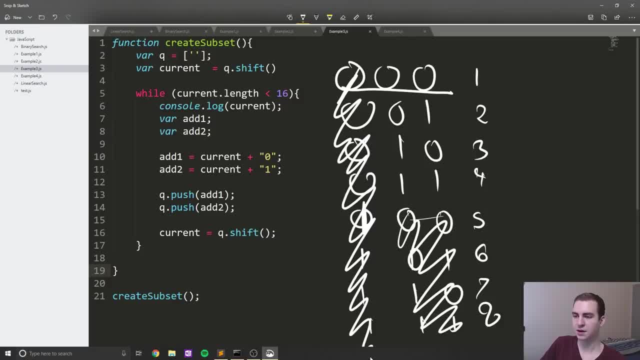 look like these: 000.. So these are all the same as the ones above. So we get four. So for two digits we get four. for three digits we get eight. for four, we get 16. And we essentially get two to the amount of digits. So in this case we get to the 16.. So that takes a really 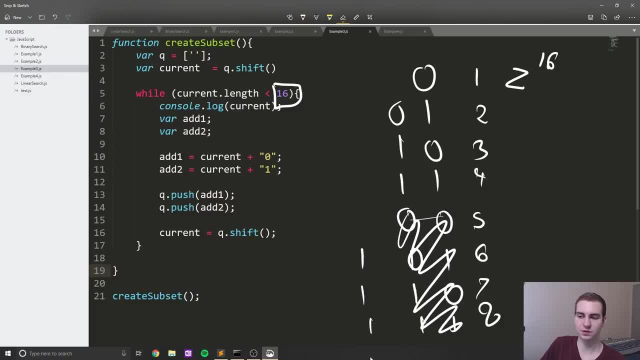 long time to run right Our input size. It was only 16, because we're only doing 16 digits. But two to the 16 is a massive number And that's why it took us so long to run that program. So you know, if we had had an algorithm. 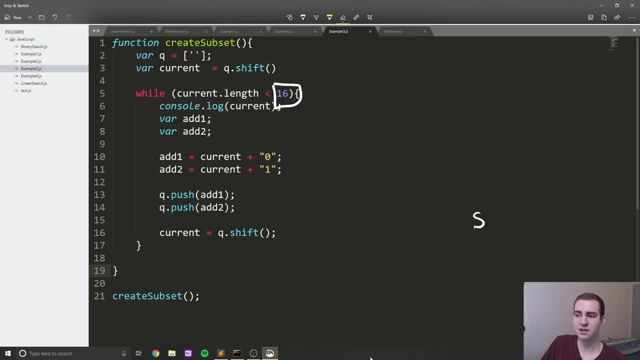 that could do that in linear time, then we would only have ran it 16 times And that would have happened instantly. But it was happening in two to the 16, which means that it took a long time, And that's another reason. obviously we need to understand time complexity. 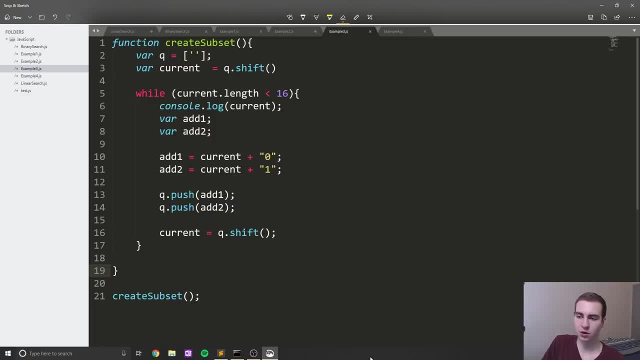 and how long these things are taking. Now again, notice, right, like I'm doing all of this stuff in this loop, like I'm doing 12345678.. operations every loop, And this loop is going to happen. Well, two to the 16 times, okay. 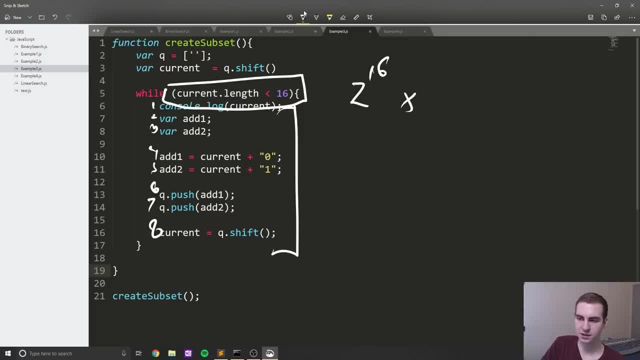 this happens to the 16 times multiplied by how many operations is this eight? Now here's the thing, right, like two to the 16 is a massive, massive number. multiplying it by eight, yeah, it makes it eight times larger, But really like we can just neglect this. 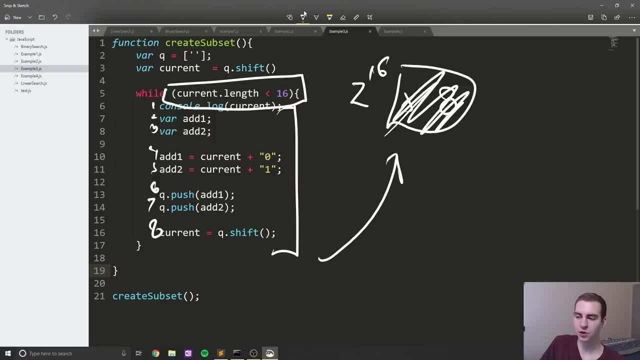 because it doesn't really tell us anything more. But the shape: we know the shape is exponential and it's happening like very taken a really long time. Multiplying it by eight doesn't really give us much value, It just kind of tells us it's. 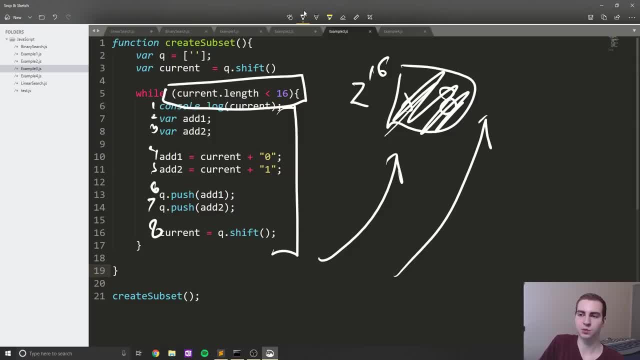 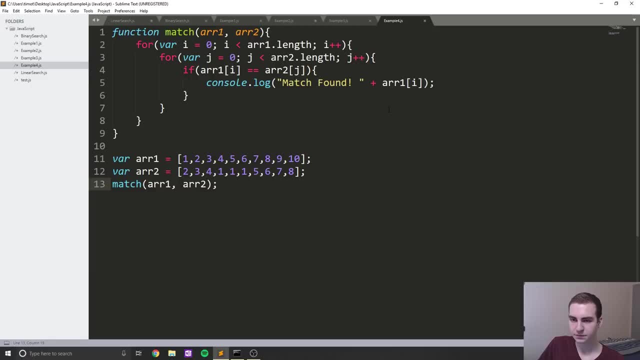 eight times larger. It doesn't tell us the shape of the increase, which is what we care about. We just care about the shape increase. Okay, so that's kind of it for that one. What was the other example I did? Okay, so this is one with two input variables. we're going. 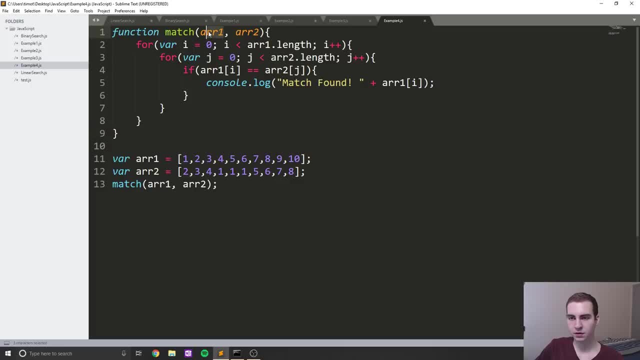 to talk about now. Now we do this Alright, so we have array one and array two. Now, how do we do this with two input variables? Well, essentially what we do is we just say: we're gonna look at the first for loop, we're gonna look at the second for loop, And then 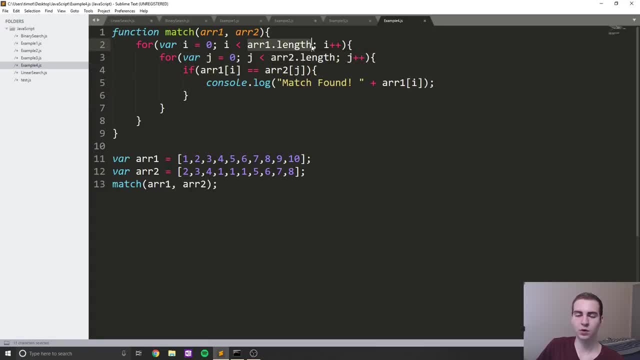 we'll just see what happens in here. And this first for loop. well, what, what does this run? Well, this runs in length one, okay, so like, array one has length of n one, array two has length of n two. So this first for loop is going to happen. what? and one times. 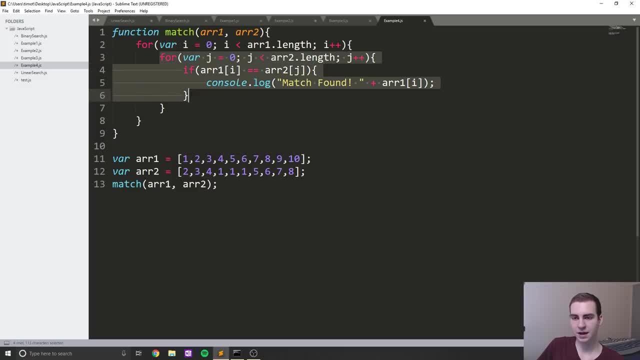 and this for loop. the second for loop happens, and two times, but it happens every time that n one happens, So we say this happens and one, this happens and two. So since this for loops inside of the other for loop, we simply say this is happening in n one. 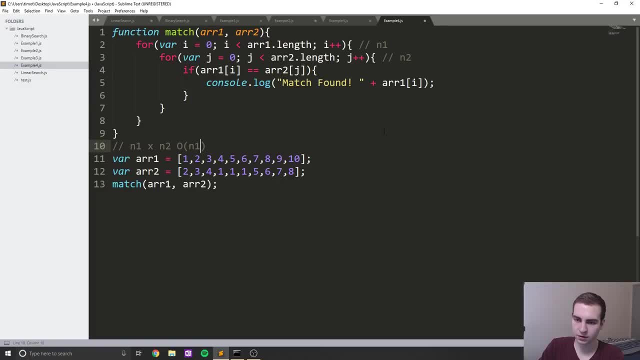 Times and two time, in other words big O of n one times and two, And that's how we determine that. So this runs in n one times, n two, And the reason we can't just simplify this is because obviously these variables are different, And with this list was like 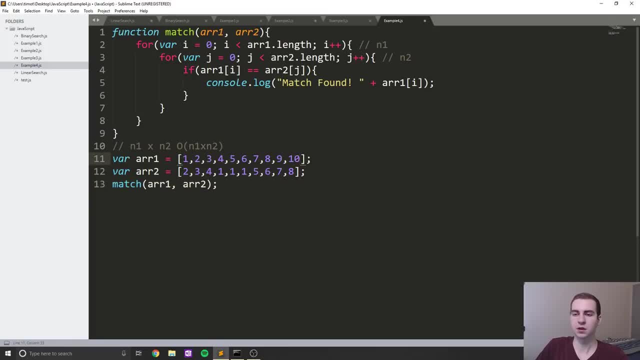 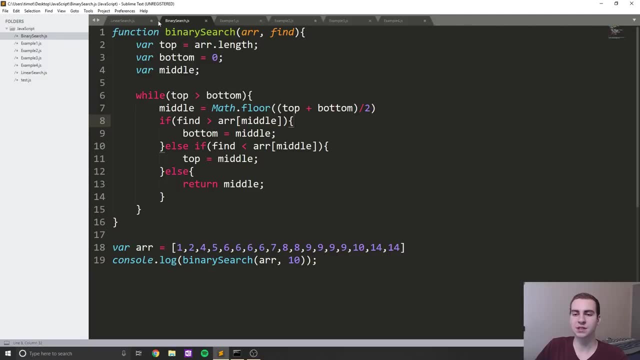 way bigger than the other one, it would affect how long it was going to take. So yeah, so that is kind of been it For bigger notation introduction. I hope that you guys at least have some sense of kind of the speed of some different algorithms, how you can kind of 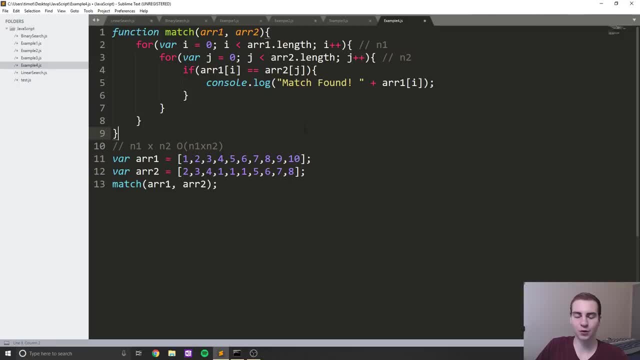 look at them and get in that A very brief idea of how long they're going to take. this is super useful And I highly encourage you guys to be critical of yourself if you're writing efficient code or not. If you're writing code that runs in n squared, just know it's going to take a long time to. 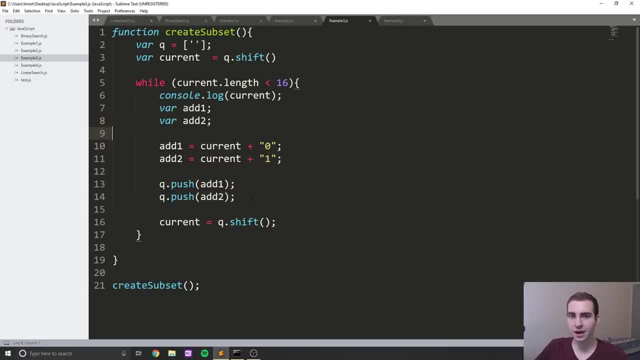 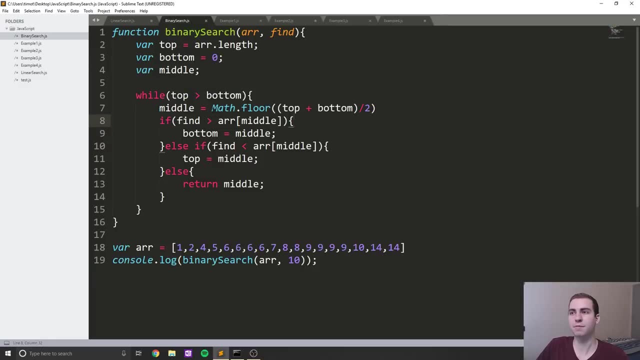 run right. If you're writing something like this that happens in two to the end, understand that that's going to take a massive amount of time to run, And if you're writing something like binary search, you're going to be like, well, if I have massive lists, it might make. 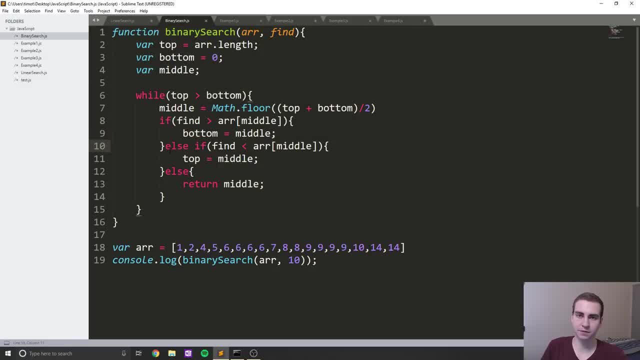 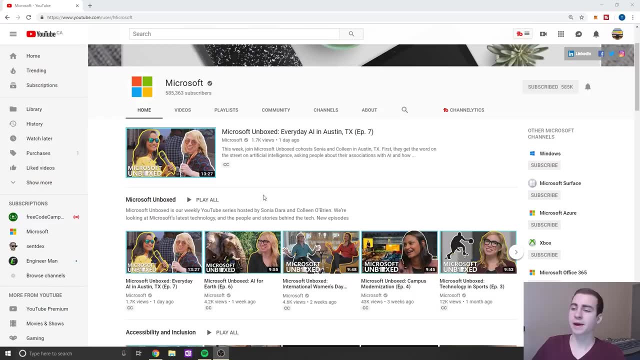 sense to use a binary search on them, because it can be so much faster to find elements right. So, as I wrap up this video, just a reminder that this video was sponsored by Microsoft. if you're not already, you guys should head over to their YouTube channel.